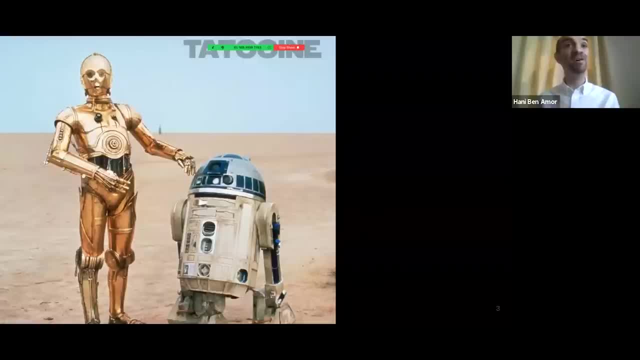 movies were shot in Tunisia in this place called Tatawin, just a couple miles away from me, And so growing up, I had this impression and vision that robots would be roaming up and down the streets just a couple miles away from me. And what's really compelling about the vision of the Star? 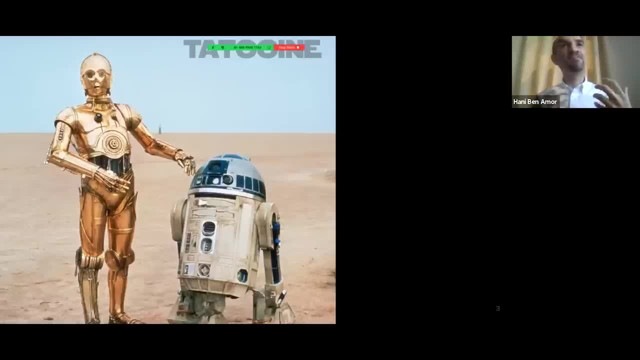 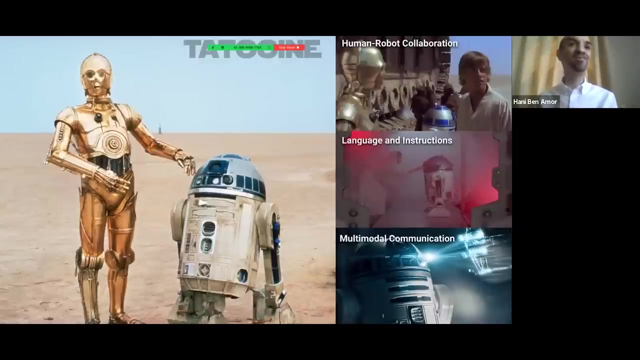 Wars movies is this vision and the kind of really enthralling vision of humans and robots working together, And I think that's really important And I think that's really important, And I think that's very important, And I think that's really important, And I think that's, And I think that's. 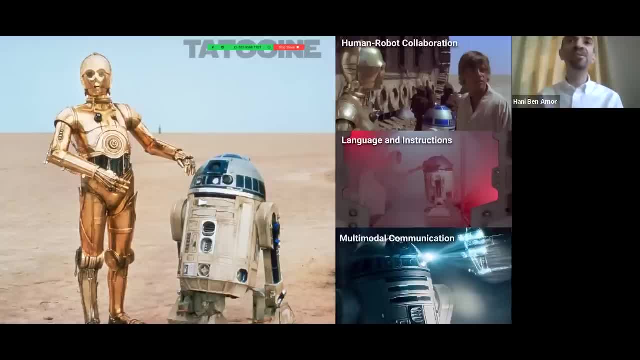 very interesting. we have a lot of viewers who see this as a sort of Yahoo button that you see the name which resto失 omo. So on one hand it shows human robot physical collaboration, so they share the same physical space and they engage in physical interactions with each other. 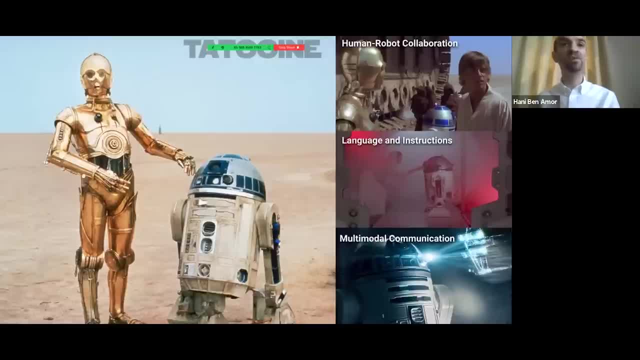 But at the same time we're also seeing interactions through language and instructions. So, most famously, in one of the major scenes of the movie trilogy, Princess Leia gives the robot R2D2 instructions regarding the Death Star by just talking to the robot. 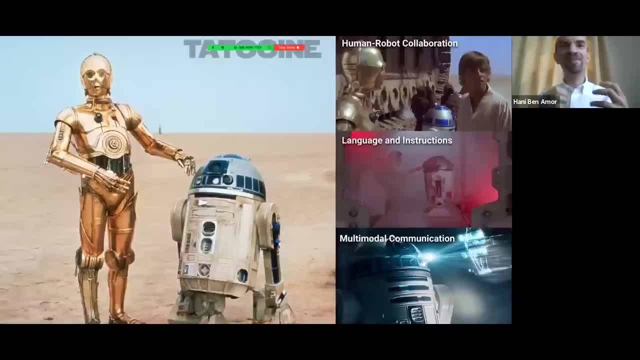 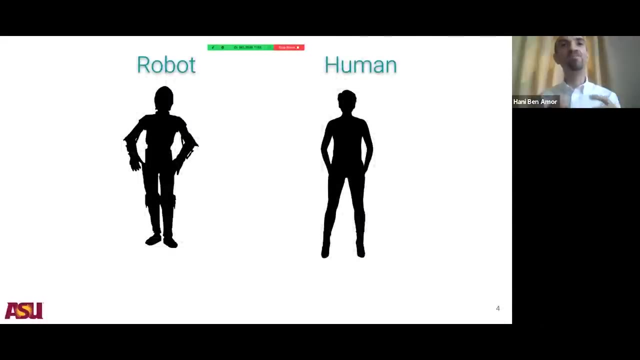 But at the same time, the movies also showed really new and innovative ways of communication and collaboration. So, for example, the R2D2 robot is able to use holographs and projections to communicate with human partners, And that's exactly the kind of stuff that I'm interested in. How can we bring humans and robots together in shared physical spaces such that they become partners? 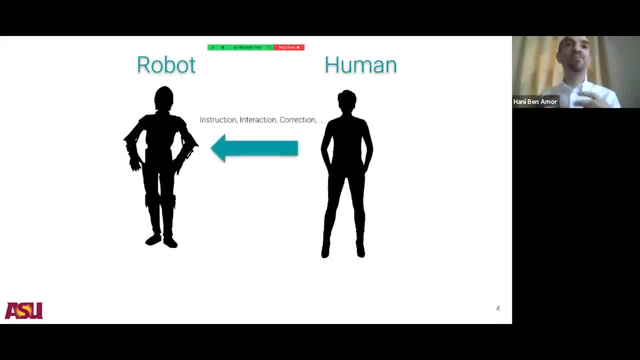 And so, for that, what we need to be able to do is to enable the human To interact with the robot. so, for example, provide instructions, provide physical interaction, maybe even correction, saying hey, this is not how you do it, this is how you do it. 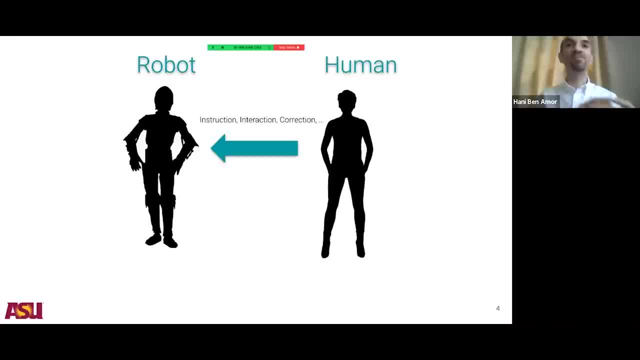 So there is some information flow from the human to the robot. But for this to be a true partnership, we also need the other way around. we need robots to be able to communicate back to humans. So, for example, a robot may be providing an explanation saying why it did something. 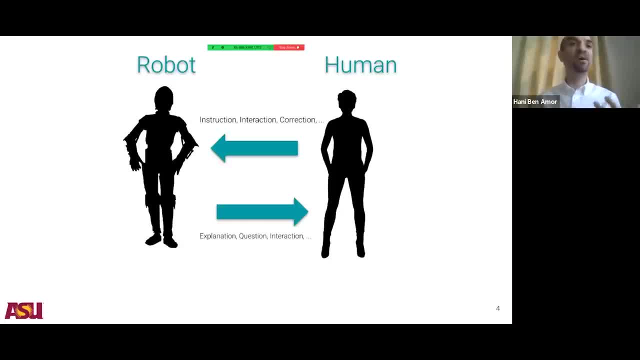 Similarly, a robot may ask the robot. A robot may ask a question to a human sort of a clarification And, of course, in all of this the robot needs to be able to physically engage and interact with the human partner in a safe manner. 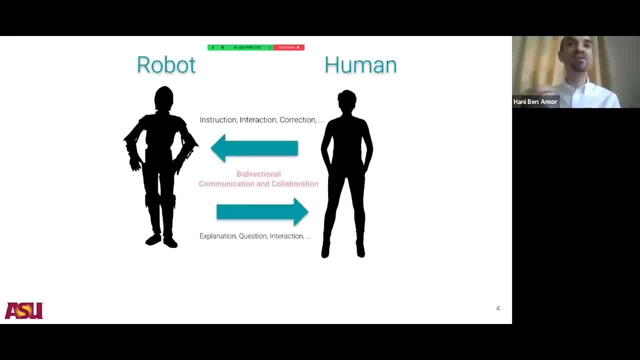 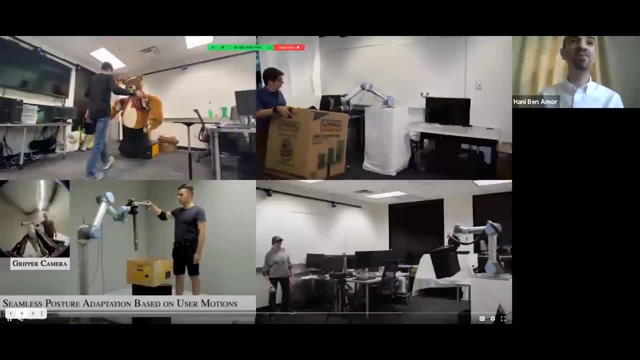 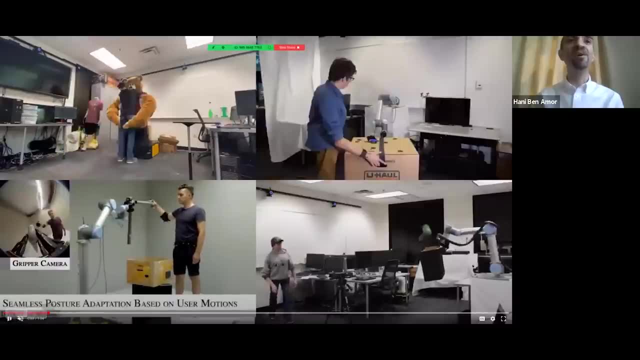 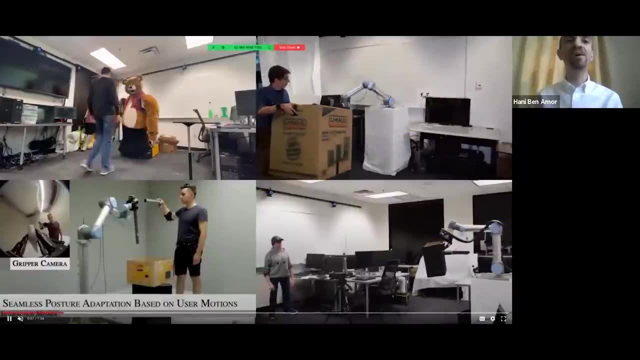 So we built and develop new machine learning algorithms for robots that allows them to physically interact with human partners. So think of, for example, the robot that learns to hug you, a robot that learns to do assembly with you, or a robot that learns to so here in the corner, a robot that learns to catch a ball with you. 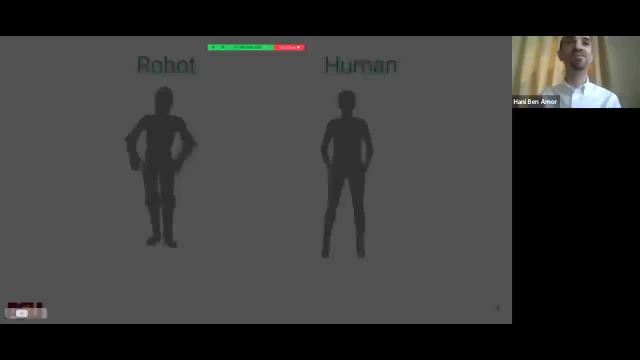 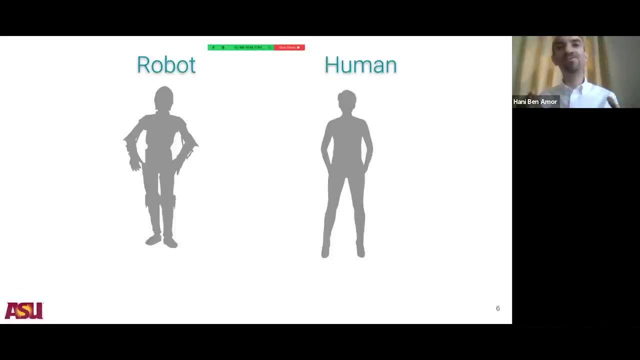 And so just generally, humans and robots working together on some complex physical tasks and communicating with each other. And, of course, as I mentioned earlier, this is a rather big theme and it has multiple manifestations. What I'll be talking about in this talk is three specific things. 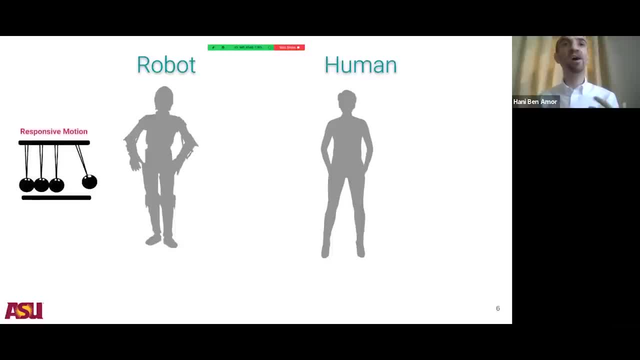 So the beginning of my talk I'll be talking about responsive motion. how can robots create and generate responsive motion that is adaptive to the human's needs? Similarly, for humans and robots to work together, they need to synchronize their time. In many domains we say timing is everything, and if you get the timing wrong, nothing works. 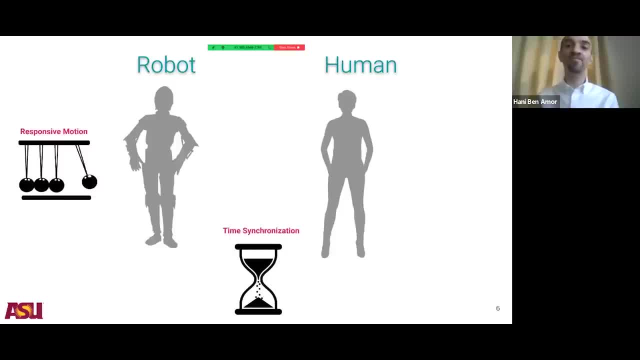 And so how can we synchronize timing between these two partners? And finally, I'll also be talking about communication and the role of language in this sort of partnership and collaboration, And what I mean by language is not only natural language, but also other forms of language, such as pictorial language. 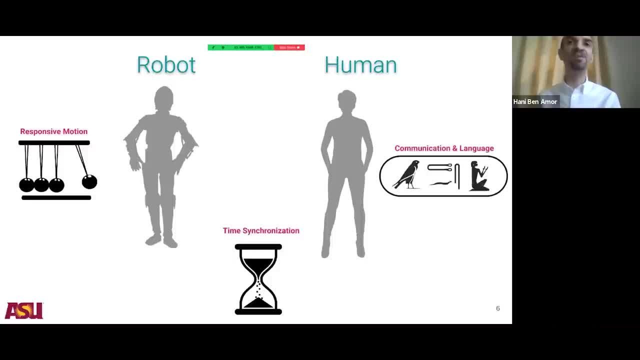 Think, for example, about the hieroglyphs in Egypt. that's a sort of pictorial language, And so with that we come to the outline of my talk, And I shamelessly struck to the point where I said I don't want to talk about language. 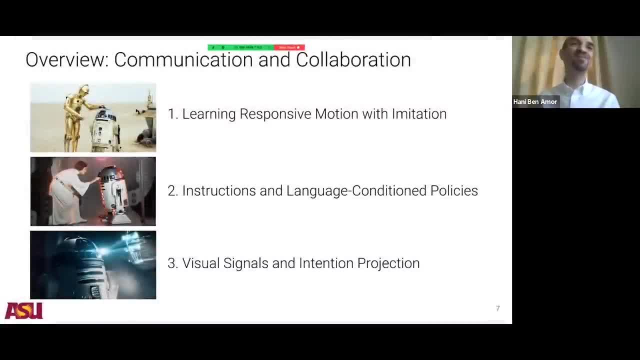 I shamelessly structured my talk along the scenes from the original Star Wars trilogy, So in the beginning I'll be talking about learning responsive motion with imitation. After that we will focus on instructions and how we can use natural language to create language conditioned policies for robots. 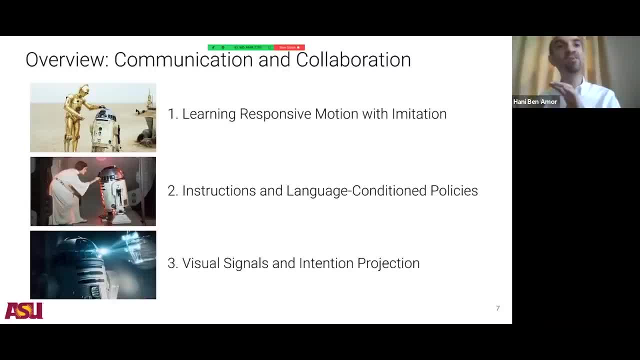 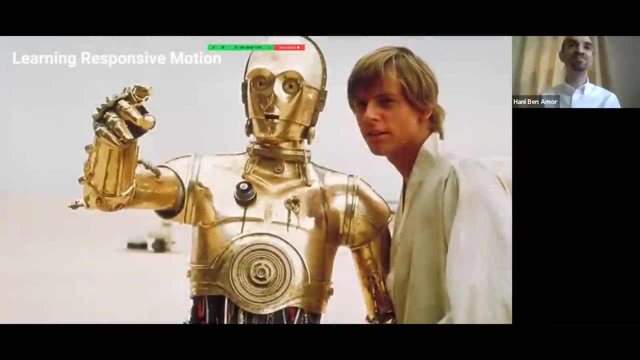 And, finally, we will switch gears and focus on how the robot can communicate back to a human partner. And so there, we will focus on visual signaling And intention prediction. Okay, without further ado, let's start with the first part: learning responsive motion. 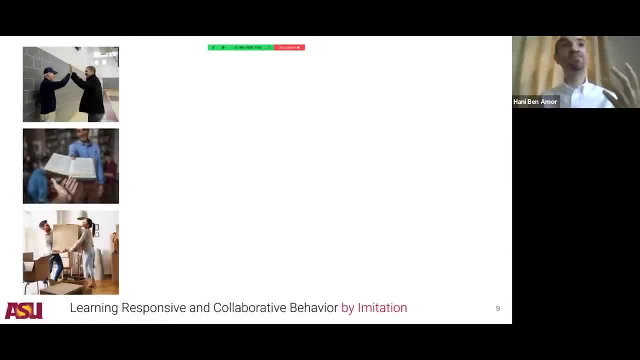 So what do we mean exactly by responsive motion? Here are a couple of examples. Think, for example, about the person high fiving someone else, or a person handing over a book to someone. Similarly also collaborative lifting of a heavy box. In all of these scenarios we have some sort of social interaction between two partners. 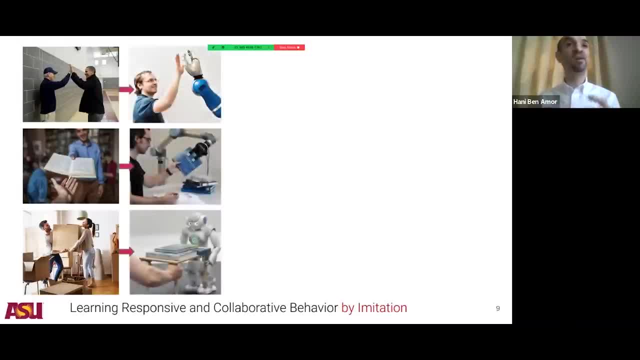 And what we'd like to do Is to copy that and be able to create robot controllers that allow robots to engage in similar interactions- physical and social interactions- with human partners. So a robot that high fives you or helps you carry a table, for example. 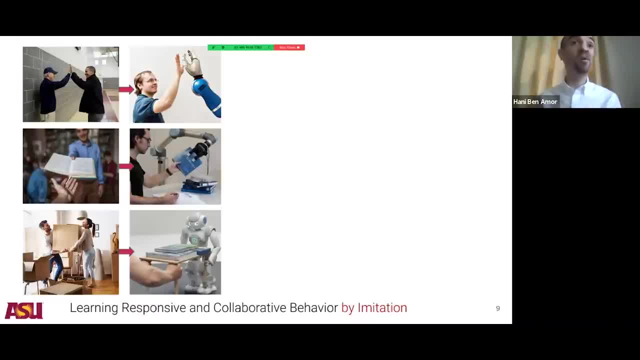 Now programming. this is rather arduous and complex. It's very hard to predict what the human is going to do, And the methodology that we're going to propose in this talk is to learn these sort of collaborative and social behaviors through imitation. 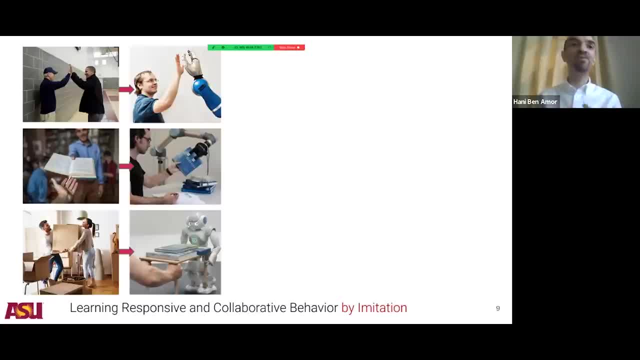 So by observing people. So think, for example, about the following scenario: Imagine you have a robot that is sitting in a park bench in a park on the first day. It's just observing how people are high fiving each other. So it's observing multiple people high fiving each other. 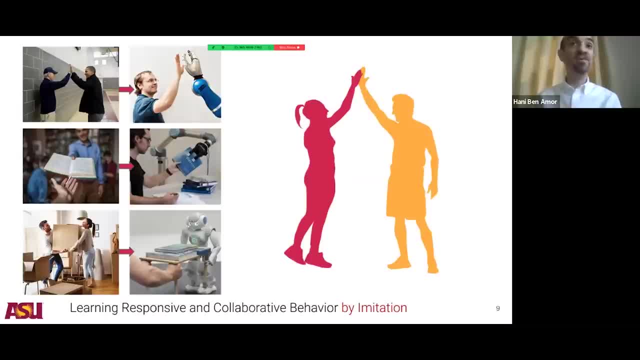 Can the same robot on the next day go in there and engage in a similar interaction? So what the robot would need to do is to learn the rules of engagement, You could say to learn from these examples how and when to engage in such an interaction and how to adapt the hand position, for example, and the timing to the human interaction. 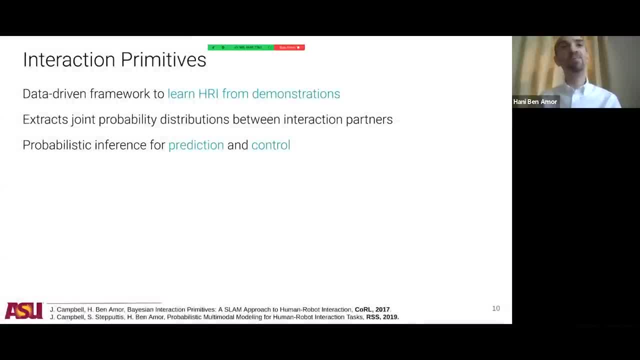 And so, in order to realize that, a couple of years ago we proposed a framework called interaction primitives, and it's a data driven framework that allows robots to learn HRI. so human robot interaction from demonstrations. The underlying principles are really simple. So first we have videos or any sort of demonstrations of how people engage with each other. 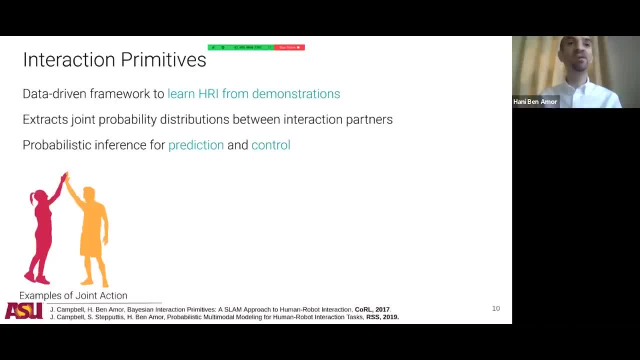 And now from that data we extract the information to model the mutual relationship between the two interaction partners, So person A and person B, And we model this as a joint probability distribution. So we have a probability distribution that models how did person A adapt its movements to person B and vice versa. 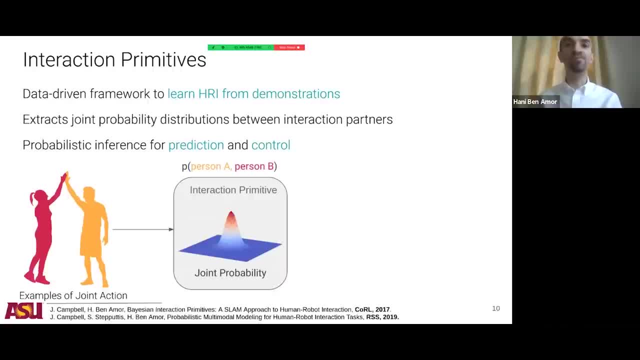 And this joint probability distribution is called an interaction primitives. Once we've extracted it, we can then condition on it. so basically perform Bayesian inference, We can condition on it and say: well, now a robot is seeing a new person, or the same person engaging in a new interaction. 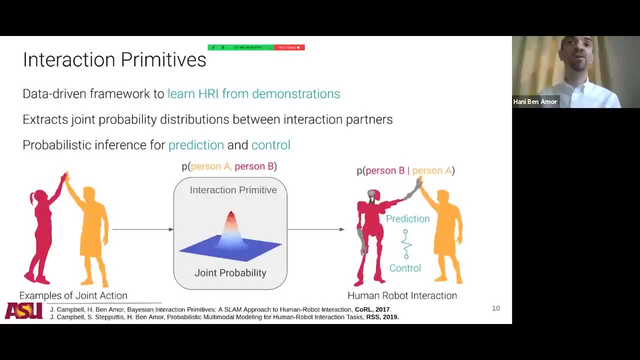 And now it conditions on that interaction and gets back the conditional probability distribution that tells it what would person B have done in this scenario, And so once we have this conditional probability distribution, we can use it for control. But one thing that's really nice about this framework is that it actually encapsulates both prediction and control within the same probabilistic framework. 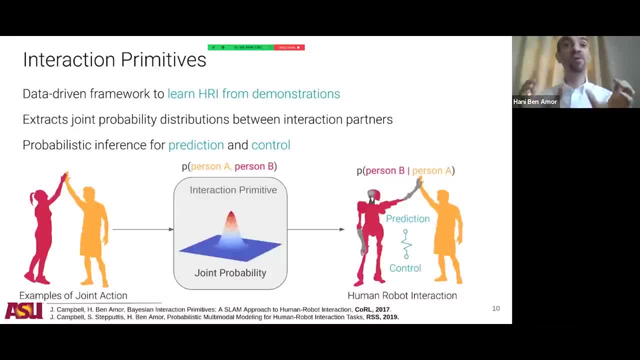 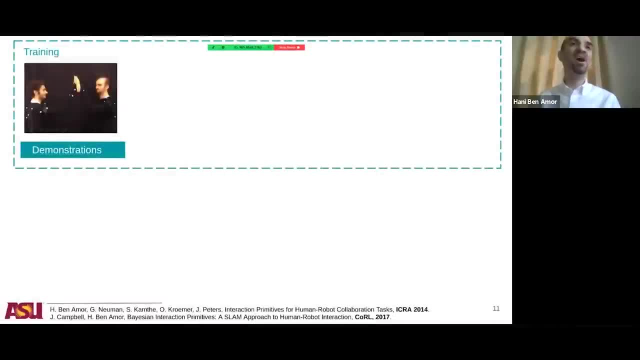 So, instead of having two boxes, one for prediction and one for control, both of these are integrated and are two sides of the same coin. Now, how do we actually do this? Well, for example, let's take the high-five demonstration and the high-five task. 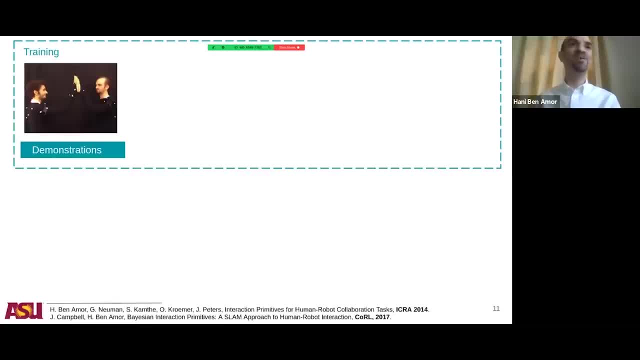 So here's a picture of me and my partner. This is my former student Marco. We are in the motion capture lab and we're just recording our own motion. So once we've recorded these demonstrations of multiple high-fives, we then represent the observed trajectories, so the recorded data, in a certain fashion. 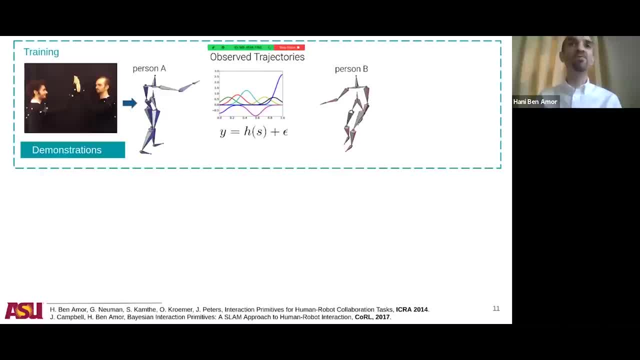 And we represent the data y. so that's what we recorded. We represent it as a function h of some latent state s plus noise epsilon, And we'll talk about this later a little bit more in detail. But the underlying idea is to have a compressed representation from which we still need to be able to extract the component sA for person A and the component sB for person B. 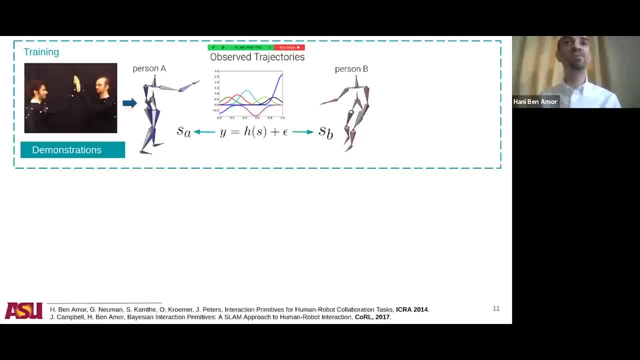 So this compressed representation should still allow us to extract out of that the components for each one of the partners. The interesting and novel part here is having this function h of s, which is a function of a latent state s. So s is our latent state representation. 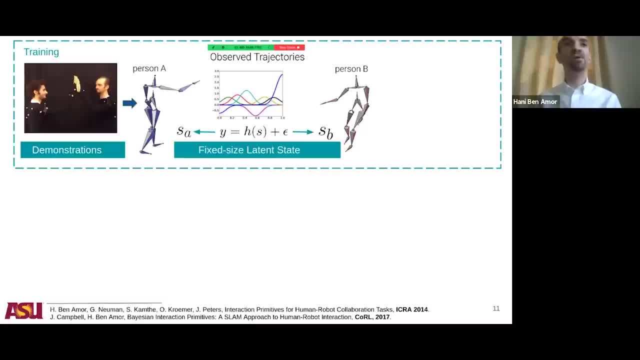 And so the second state is our latent state representation. And so the second state is our latent state representation. And so the second step in our framework is to bring the demonstrations to the fixed-size latent state representation. Once we've done that, we can learn a generative model over that which is the joint probability distribution I was mentioning earlier. 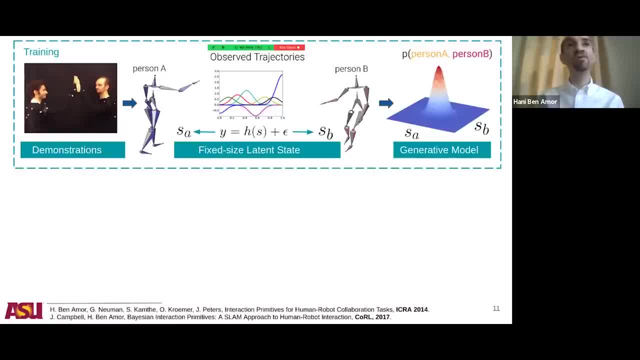 So once we have this, this generative model- so that's happening at training time, Now at test time- we can have a robot engage in a similar interaction. So the robot sees a partial interaction, meaning a partial movement of the robot. 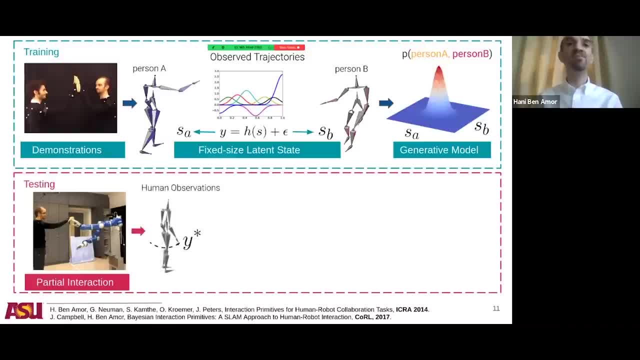 So the robot sees a partial interaction, meaning a partial movement of the human interaction partner. So, for example, the person may be just starting to lift the hand, And so that gives us a new data set, y star. What we can do is to condition on that. 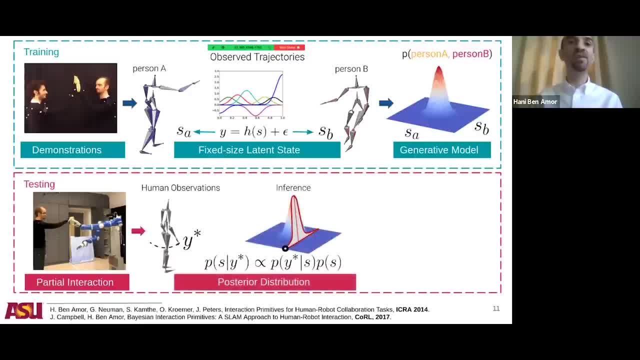 And so we have a probability distribution over the latent states, So p of s conditioned on the partial observation that we're seeing from the human. So once we've done this inference, we can then use the components of s- either s a kind of for person a or s b for person b- to do either prediction or control. 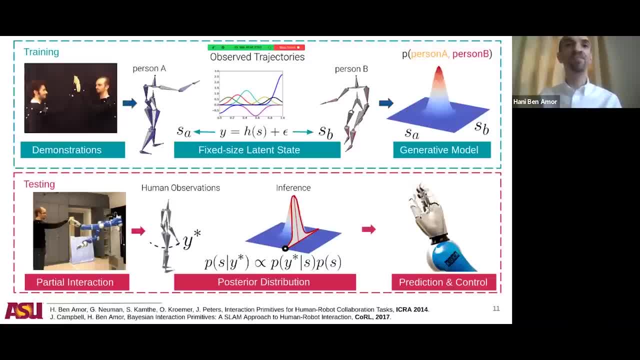 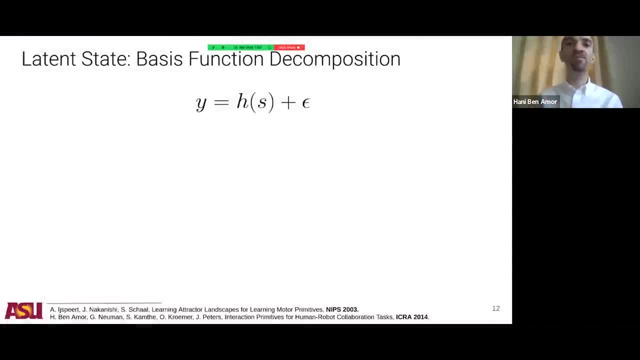 So we have both of the sides of the same coin, OK. so for this we need to better understand what the latent state representation is. So how do we actually transform our data? Well, it's actually a relatively simple trick. We take the function h of s of the latent state and we represent it as a superposition of basis functions. 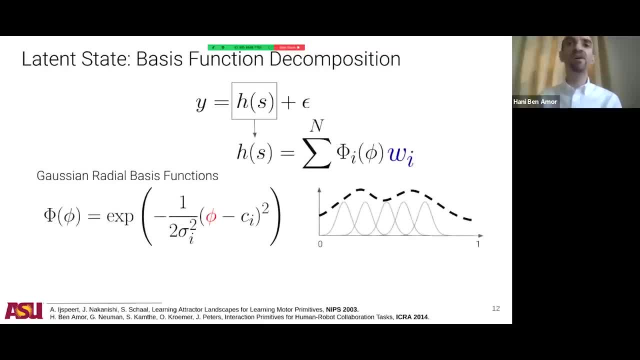 So, in other words, in this case, we have radial basis functions, That's, these gray basis functions that you see here, And what we do is we sum them up in order to approximate our trajectory, the recorded data, which is the dashed line that you see there. 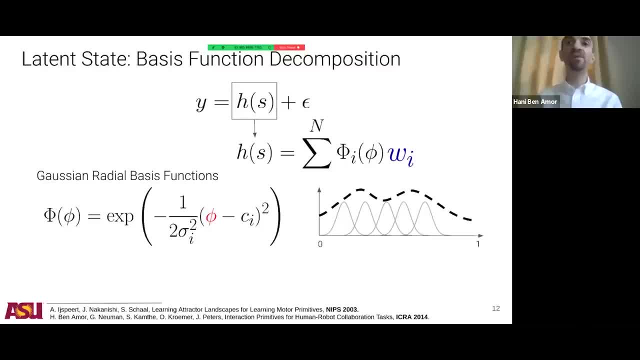 But we don't just sum them up. Each one of these radial basis functions gets multiplied by a corresponding weight, wi. So in other words, we're just doing radial basis function approximation here. But the moment we do this, we're also introducing a new variable into this, which is phi. 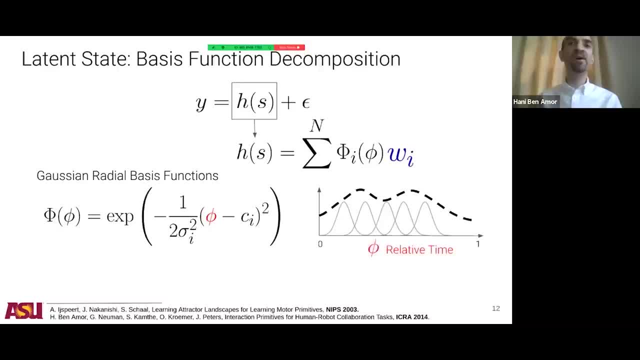 And the variable phi can be seen as a relative timer. So in other words, this is just a phase variable. When the relative time of phi is at zero, we're at the beginning of the motion, And when it's at one, we're at the end of the motion. 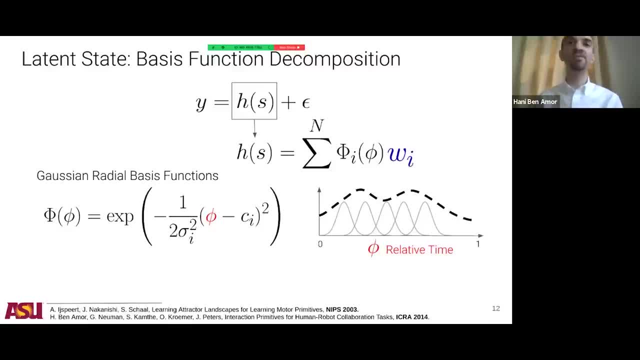 So with zero, we're just starting, With one, we're at the end. OK, so that introduces all the important components. We have the w's, We take the w's, We store them as a vector And that's going to be representing the latent state. 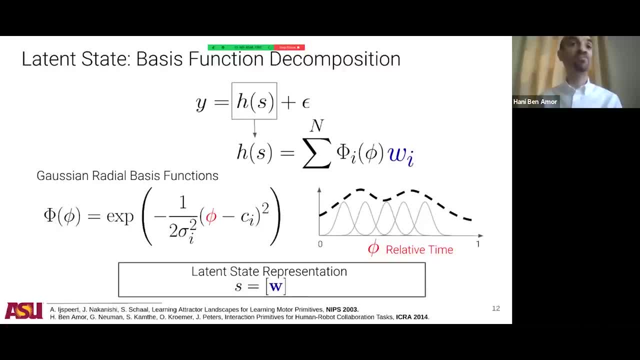 And we have phi, which represents time. So now we're good, We can just do inference over each one of these, And we should be able to do the reaction to the human partner. Well, that's what we did in the first paper. 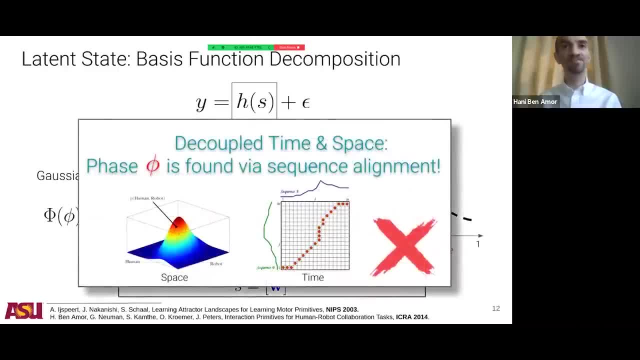 And it turned out to be a bad idea, Because the way we went about this is to use our interaction primitives and the Bayesian inference in order to model this function, In order to model the spatial part, And then we used for phi. in order to determine phi, we used time alignment techniques. 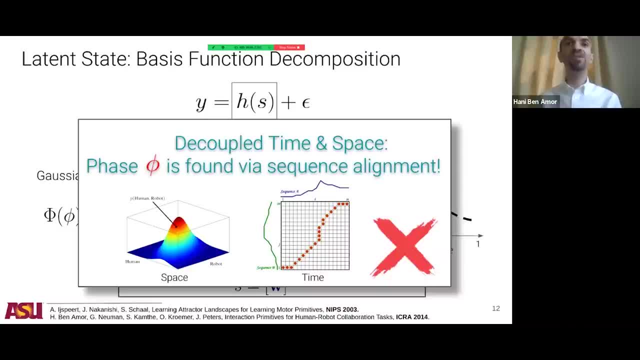 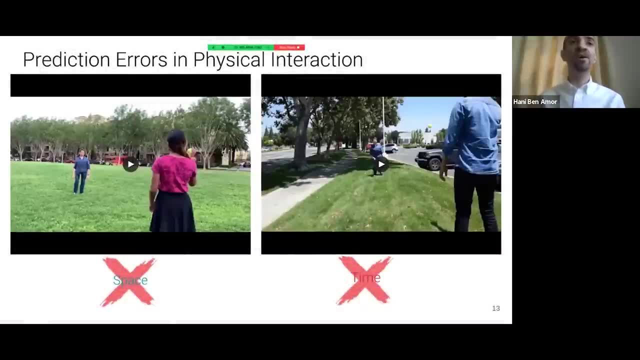 So, for example, dynamic time warping, Which, in other words, meant that we decoupled time and space, And that's not a good idea at all, And that's what we're going to be discussing now. So the reason for that is the prediction errors that you make. 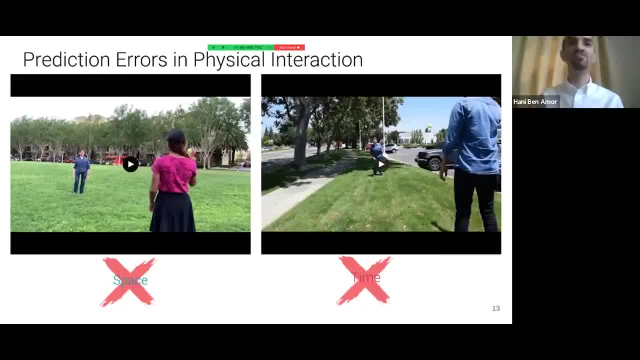 So when you're interacting with someone, let's say kind of, you're just throwing the ball and catching the ball. So that's what we see here. One kind of mistake that you can be making is a spatial mistake, Meaning the person throws the ball. 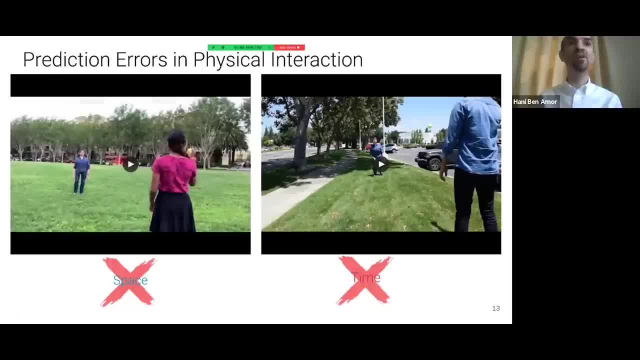 You anticipate the position wrong And, as a result of that, the collaboration fails. But there is another kind of mistake, which is the temporal mistake. And so here, in this case, my student Joe, is trying to go to the right location, but at the wrong time. 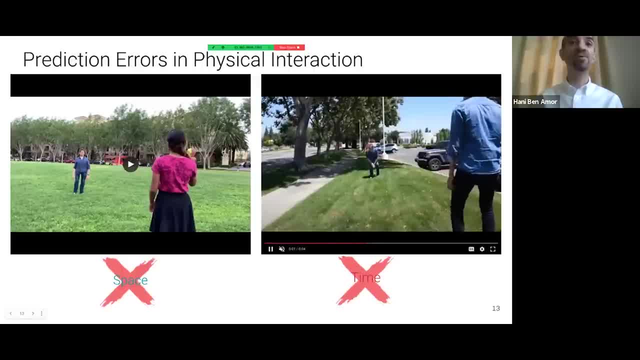 And so, as a result of that, he's not able to catch the ball. And these errors, the prediction errors in space and time, they can also be compounding each other, So if you have errors in both of these, they can become a really big error. 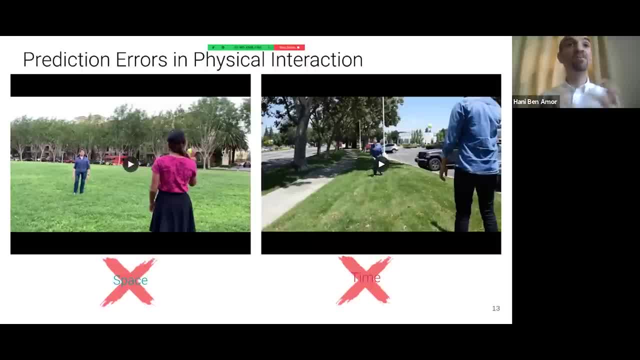 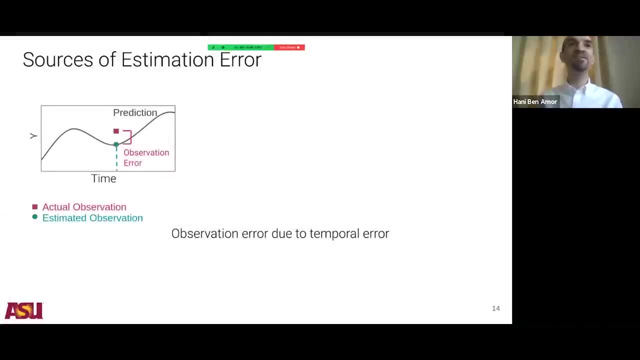 So it turns out that this is actually kind of a problem: How do these errors in time and space affect each other? But we can also use it to our advantage: how to leverage this relationship to actually make better inference. OK, let me explain this a little bit more in detail here. 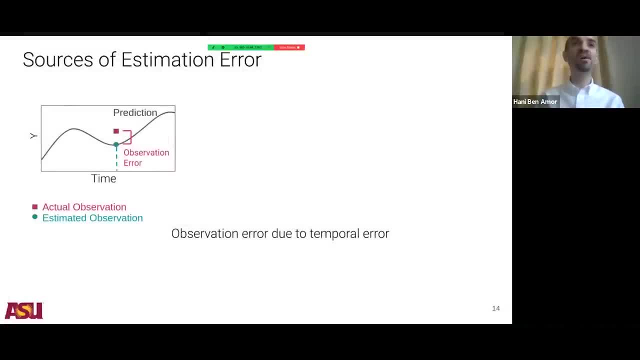 So for this we need to better understand the sources of estimation error and how to derive them and better understand them. So here you see an example. So on the x-axis you have time, So our phase variable time, And on the y-axis you have some spatial variable, spatial variable y, which could be, for example, the position of the ball. 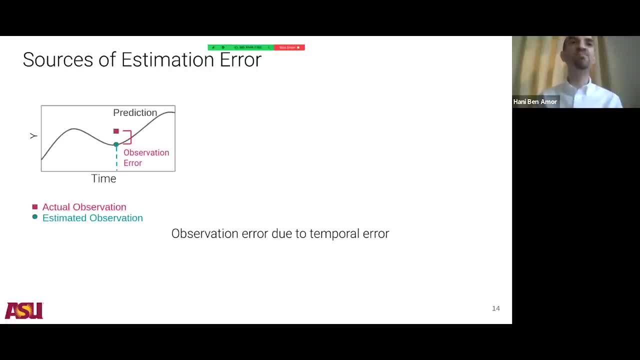 The gray trajectory that you see here is our prediction for where the ball is, And the dashed line- the dashed blue line- is our estimate of where we are in time. So, given our estimate of where we are in time and our prediction for space, we basically say: well, the blue dot there, that's where we are right now, or that's where the ball should be right now. 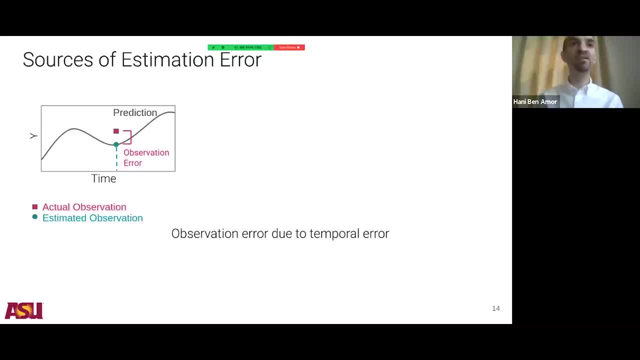 But unfortunately the camera tells us the ball is somewhere completely else. OK, the first reflex would be to say that this is a spatial error. but that doesn't have to be So. for example, this could be just a temporal error, meaning if we just shift our phase estimate backwards in time. 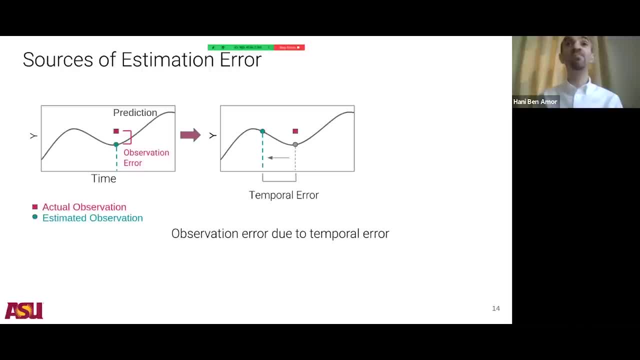 we would end up with a position, with a different position, that actually yields basically the same observation as what we see through the camera right now, But unfortunately this is ambiguous, So it could also mean that we have to push forward in time and push our phase estimate forward in time. 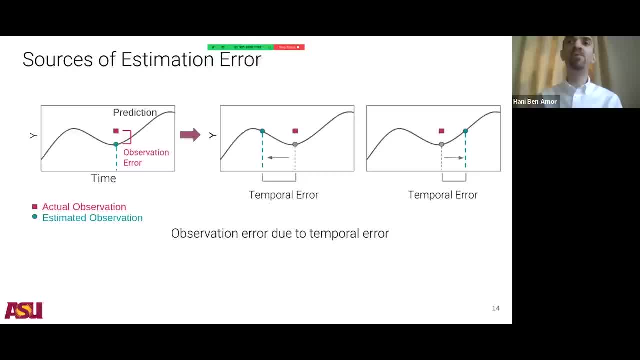 And so in that case again, we would have a new point for the estimated position for the ball which would align with our observation. So which one of these is it? If we have only a single variable, that's really hard to figure out or potentially impossible. 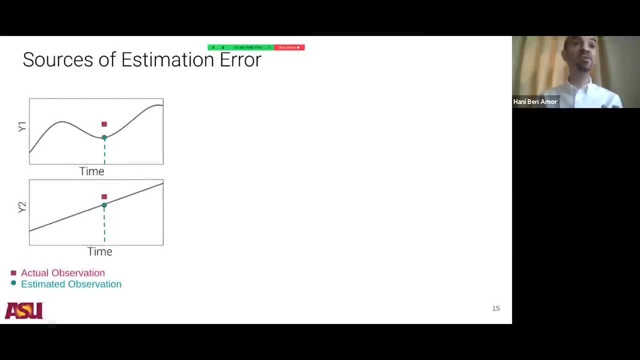 But if we use multiple dimensionalities or multiple spatial variables, we actually can figure out which one of these estimates or sources of error. it is: space or time. So imagine in this case we'd have a second spatial variable, y2. And again we have some prediction over y2 in time. 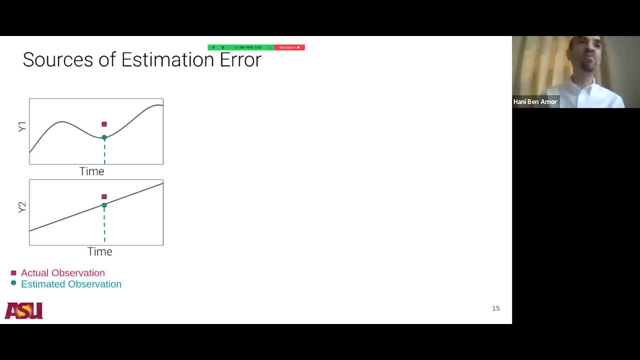 So now we have an error for both y1 and y2.. And we can try to figure out well what kind of shift in phase would reduce the error in both of these along both of these spatial dimensions. So it turns out, if we move forward in time we can reduce and eliminate the error in both of these dimensions. 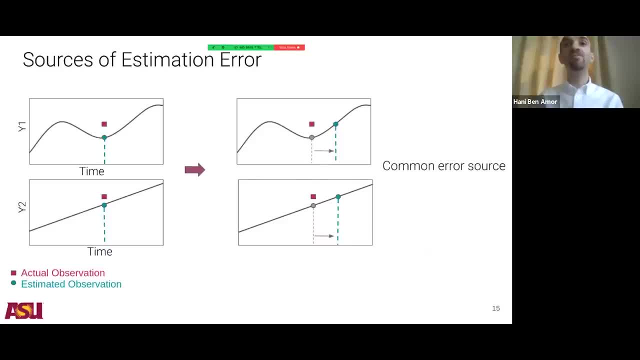 So in other words, we have a common error source here. We can leverage this information that there is a common error source and that we are making correlated observation errors. We can leverage this in order to have a better estimate of where we are in time. 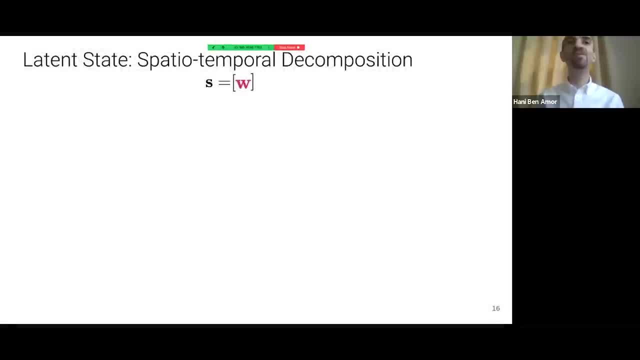 Okay, So how can we actually incorporate that into our framework? It's relatively simple. In addition to the latent variable w, we also now add phase phase velocity into our latent state, So basically where we are in time and what's the time velocity. 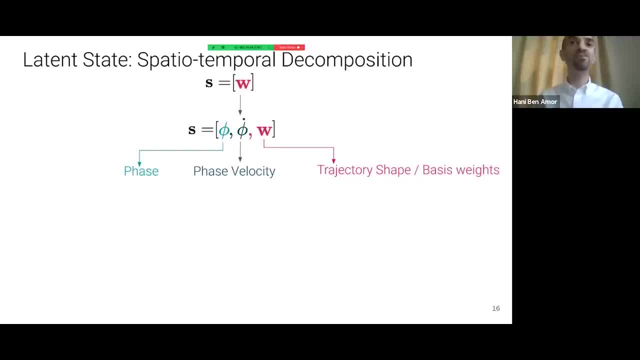 As I mentioned earlier, w basically encodes the trajectory shape, the shape of the motion, whereas phase and phase velocity models the temporal progression. One thing that's really nice about this framework is that now we can also do inference in time. So by observing a person we can also get the probability distribution over phase. 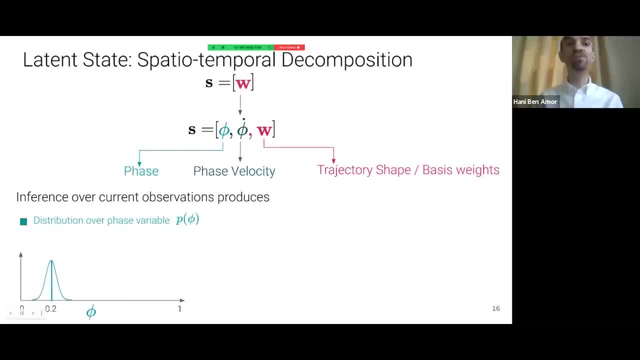 which tells us: well, it seems that we are 20% in into the motion and there is some uncertainty around it. So we have a probability distribution over phi, But at the same time we can also generate the probability distribution over w. 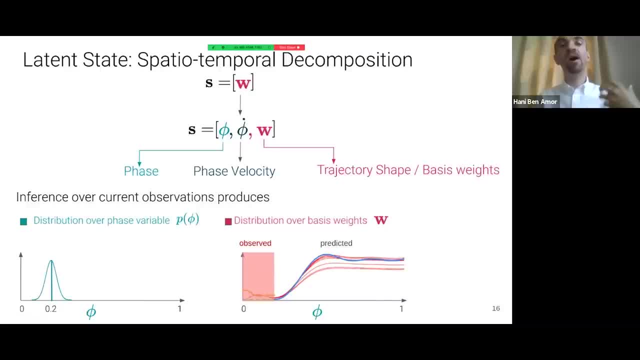 and you can think of that as a probability distribution about how the trajectories are going to continue into the future. So the prediction of the shape of the motion, And since this is a distribution, we can sample from it, which yields the red trajectories, 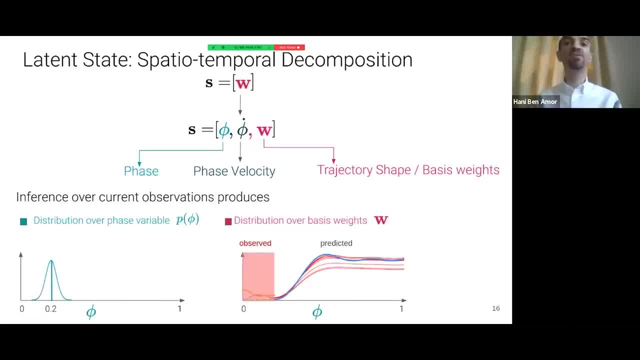 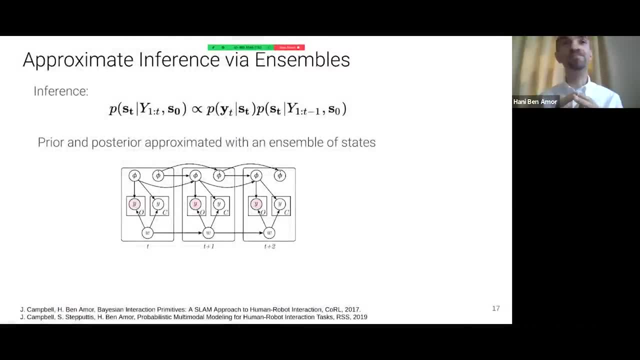 but we can also take the mean of the distribution, which is just the blue trajectory that you see there. Okay, So with all of this, let's get to the actual application. So if you're interested in the actual nuts and bolts of how to do Bayesian, 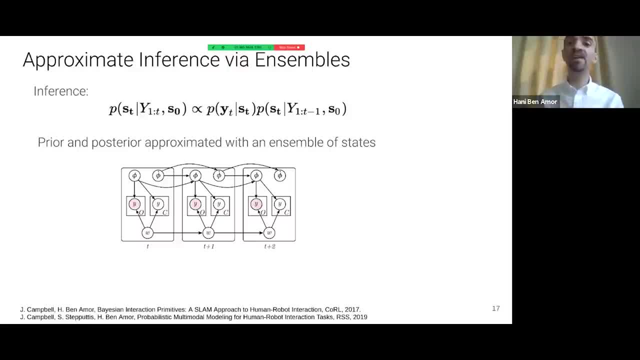 inference. here we have actually created a specific framework for that, which I'll show in a second, But ultimately, just at the high level, what we're doing is approximate inference using ensembles. So in order to approximate this posterior, the probability of ST. 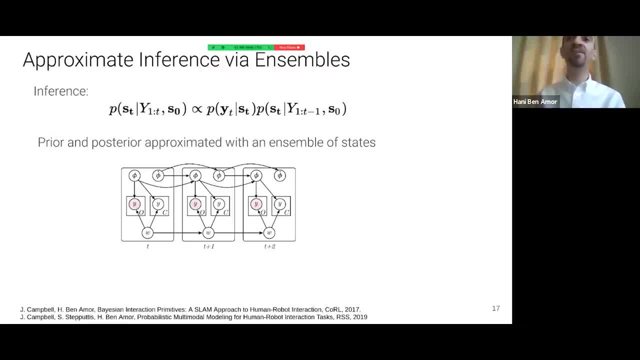 given some observations. we model that as an ensemble. as an ensemble meaning, we don't need to have any parametric assumption, We don't need to know that it's a Gaussian, for example, it could be anything- And we don't need to perform any tailor linearization. 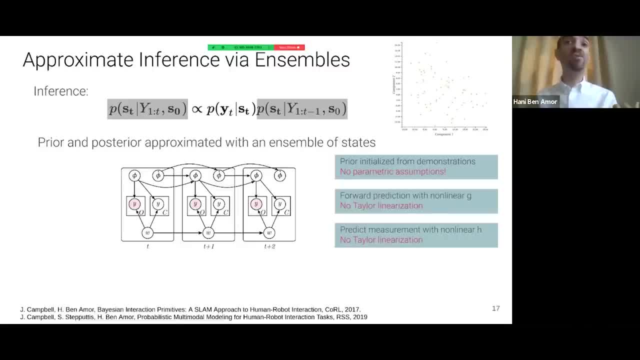 So we can make a prediction in time that is nonlinear, And also our measurements update can also be nonlinear. So within this framework we don't need to do any tailor linearization So that allows us to model these complex nonlinearities when you're collaborating with a robot or with another human person. 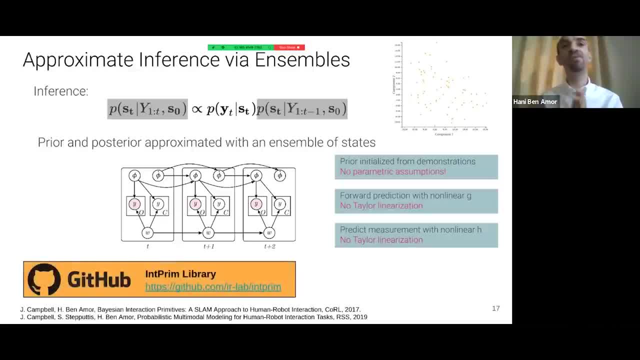 So all of this is implemented in a library called imprim, And we provide all of these inference algorithms together with a lot of tutorials. If you're interested in that, please try it out. Okay, And so with that, let's get to the 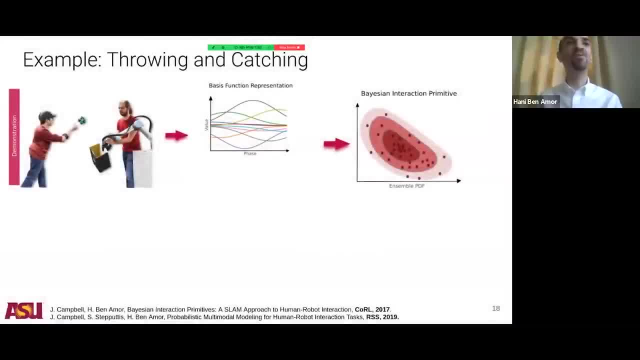 let's get back to the robotics part. So how do we use all of this? Imagine again the task of throwing and catching. So in this case we're going to have two students try to teach the robot how to catch the ball. 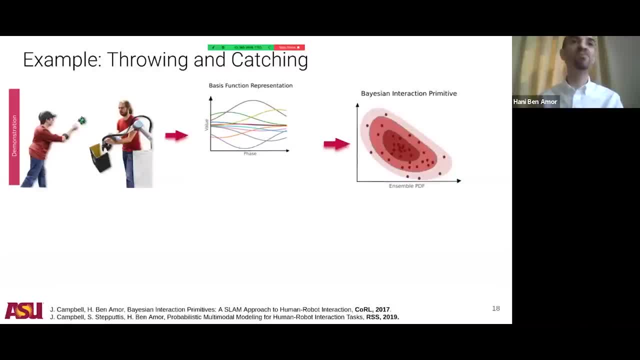 One person is throwing the ball and the other one is teaching the robot how to catch it. So we take all of this data and we learn the interaction primitive out of that, as I mentioned earlier, And then at runtime the robot can use the interaction primitive. 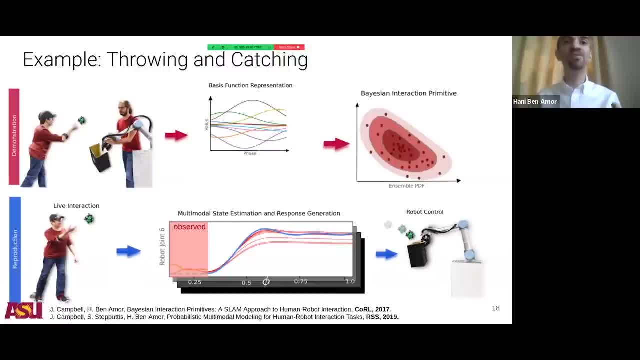 in order to make predictions about where the ball is going and where the human is going and then respond accordingly. A critical issue here. as I mentioned earlier, if we are using only a few dimensions, it's very hard to figure out what kind of an estimation error we're making. 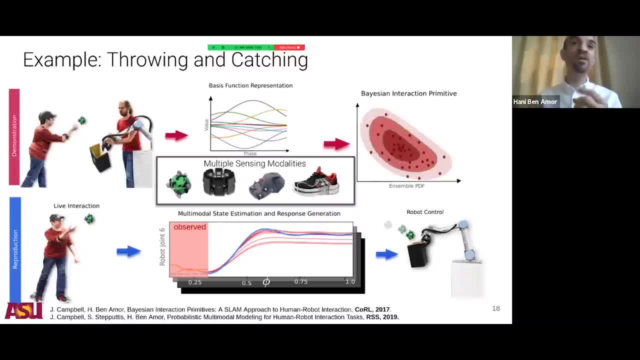 What's the estimation error source, And so what we're using here is we're using multiple sensing modalities to eliminate that error by using the multimodal capabilities of inference. Okay, So here's the actual application on the robot. The person is throwing the ball. 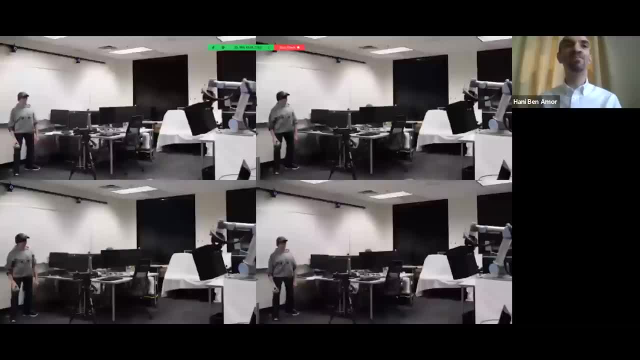 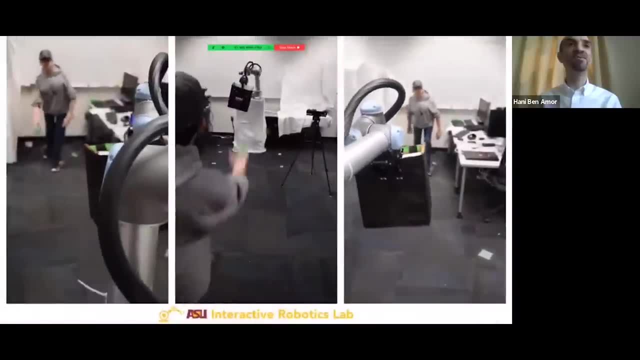 The robot is catching it And you can see the same thing again, blindfolded. now The student is throwing the ball to different locations. The robot goes there and catches it. Keep in mind: all of the robot's actions were just learned from demonstration. 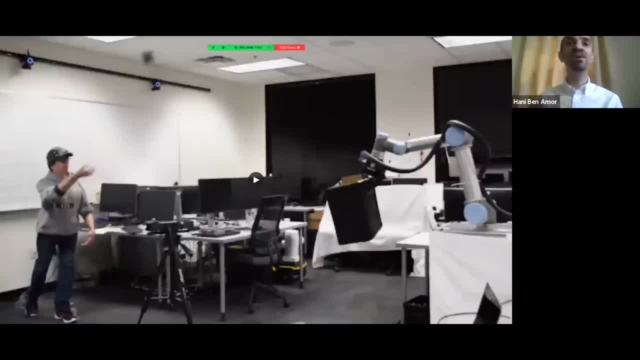 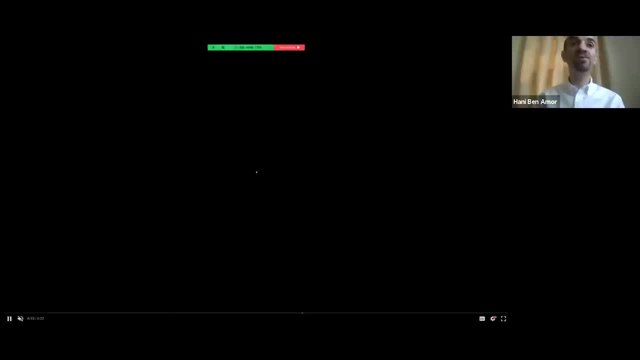 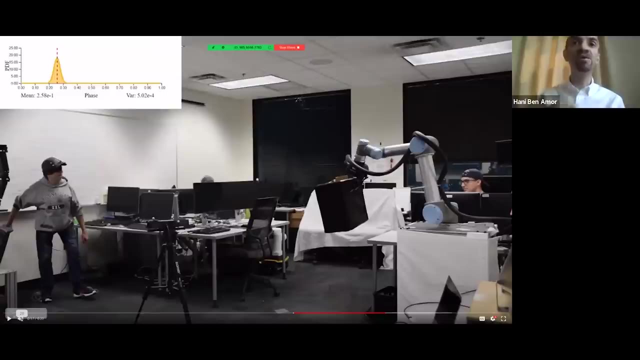 It did not do any reinforcement, learning, optimization or anything like that, It was just learning a primitive interaction, primitive, and is able to engage Well. another important estimate, or another important element here, is its ability to estimate time, As I mentioned earlier. we're actually trying to infer: 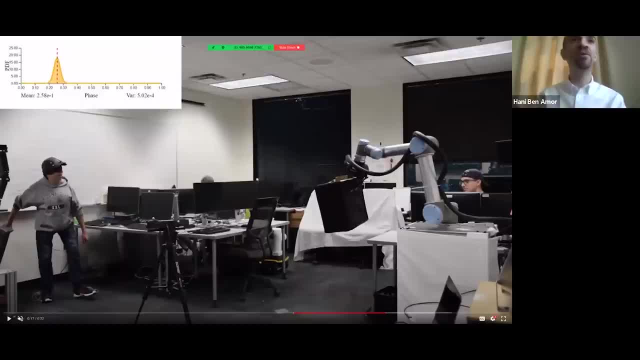 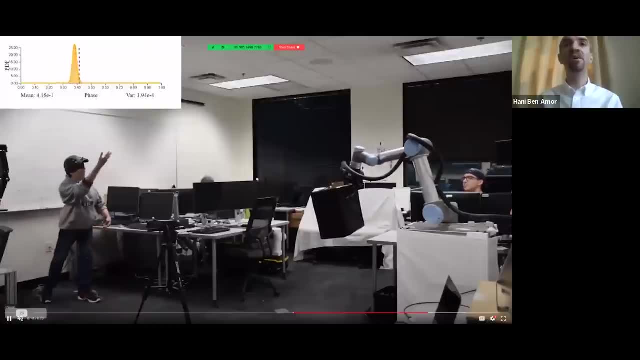 where we are in time. Are we at the beginning or are we at the end? And so that's what you see. here in the left upper corner, We have a probability distribution that gives us an estimate of where we are in time. Are we at the beginning? 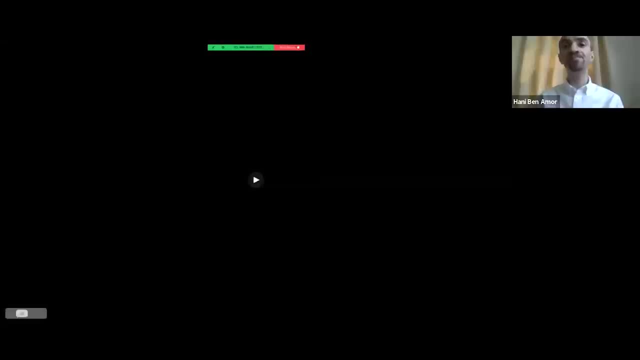 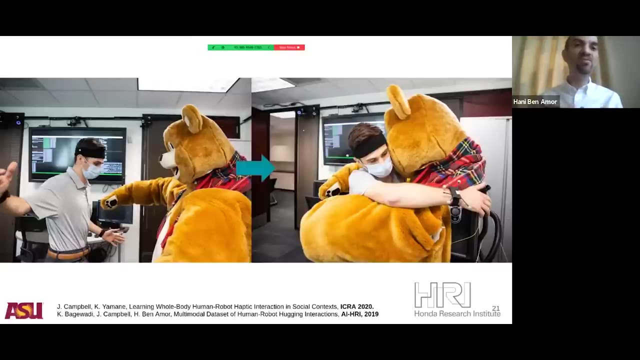 or are we at the end? So at the end we are at one, And so that's really neat. So the robot can learn to engage with the human partner. And now the question is: can we use this also for close contact collaboration? 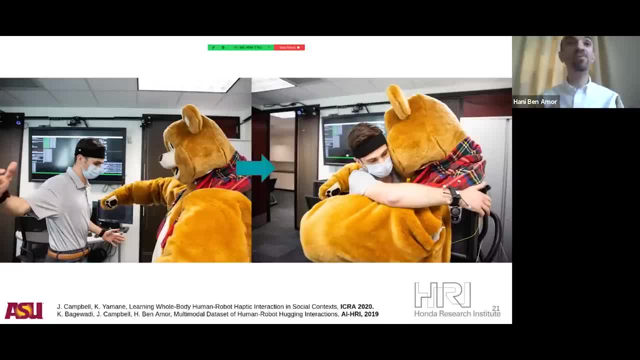 where you don't have too much of a time between the person engaging with the robot and the robot having to generate the reaction. Keep in mind also here that timing is really important. So in this case, here, what the task for the robot is is to hug a person. 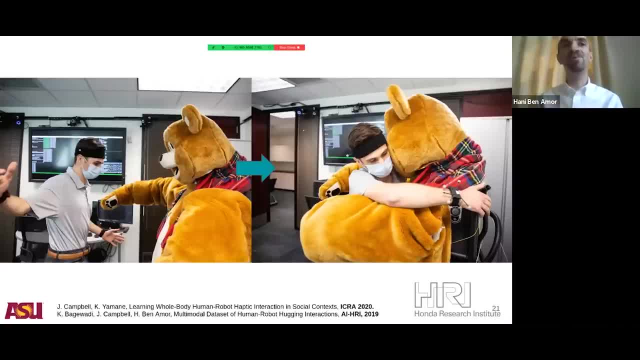 So we have here the study bear robot. It needs to learn how to hug the person And we are going to see that we use the exact same algorithms as before And the robot is trying to figure out how to hug a person, but also when. 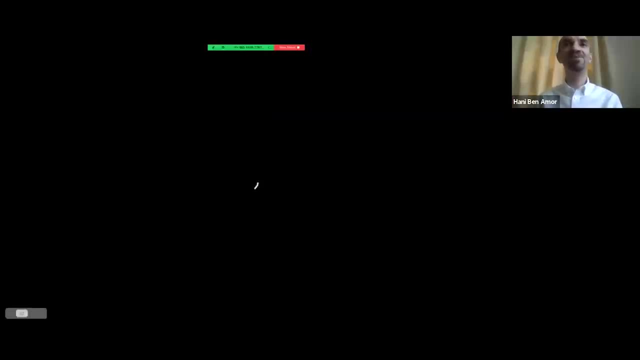 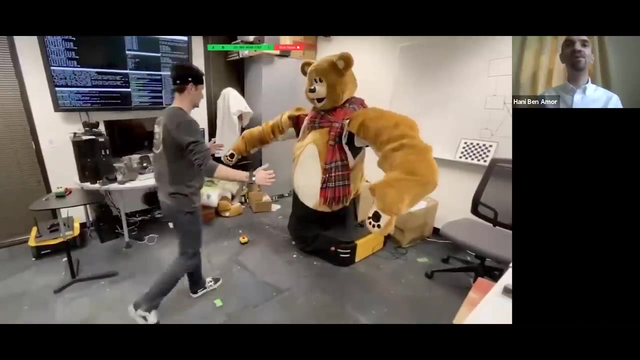 And so that's what we see here in this video. So in the beginning the person is just changing the arm positions, So the robot is adapting to that, And now it says, oh well, the person is moving in, So now it hugs the person. 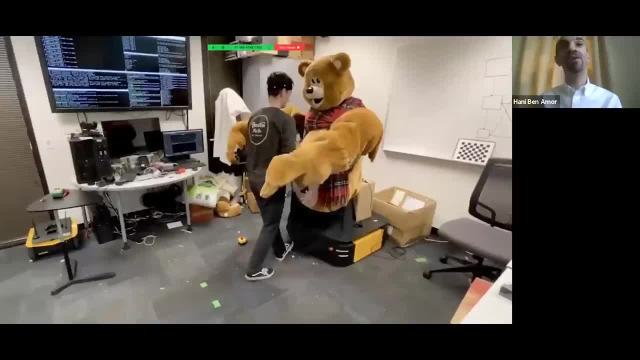 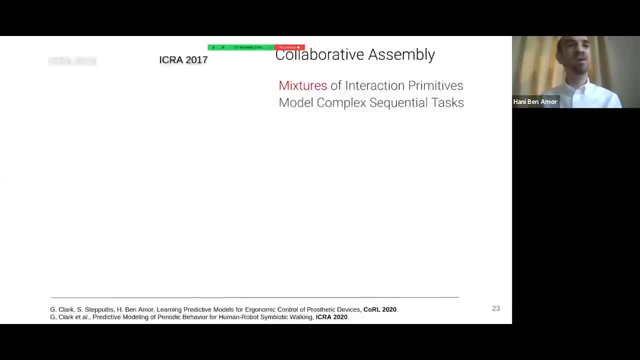 And when the person releases, the robot is also released. So here you see why spatial temporal inference is really important, incorporating time into all of this, And there are a variety of other application domains where this is true. So, for example, we use the same algorithm. 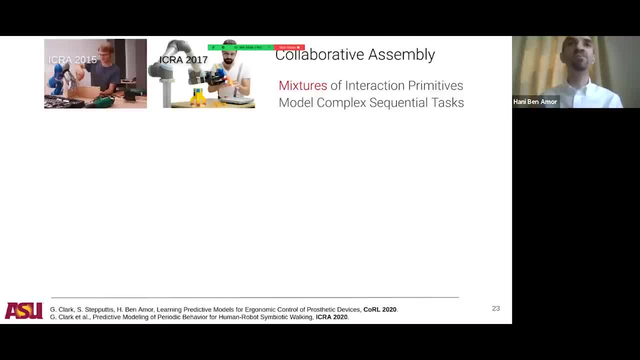 for collaborative assembly, having humans and robots assemble an IKEA shelf together. And in that framework it's not only enough to do a single primitive, We actually have to sequence multiple actions. So, for example, the robot needs to first hand over a plate. 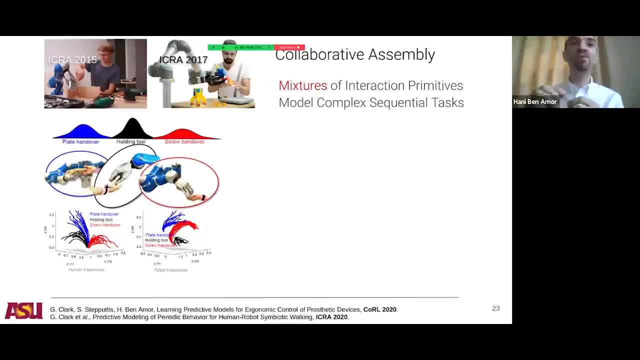 Then it needs to help a person hold the tool, or maybe hands over a screw, or maybe it stabilizes something. So, in other words, there is a sequence of actions that has to be performed there And you can actually easily show that the same framework. 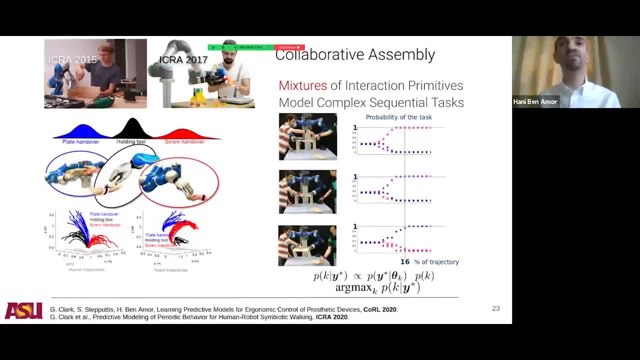 we introduced can also be used in these kind of sequential tasks where the robot has to infer in which kind of task are we right now and what should be my response. Another application domain is the ergonomic control of prosthetics. So when you're using a prosthetic, 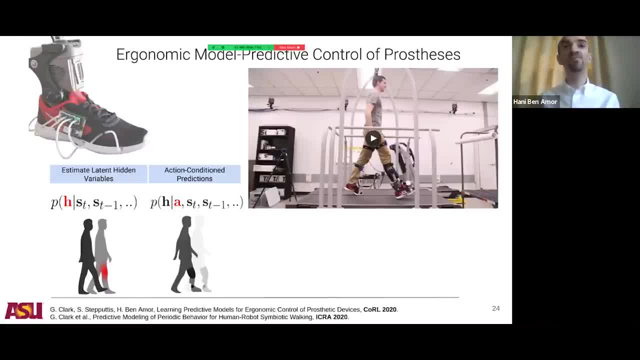 for example, it's very important that the prosthetic is responsive to the human user. In other words, this is again human robot collaboration, And if it's not responsive, then people feel awkward about it and it can actually lead to musculoskeletal diseases. 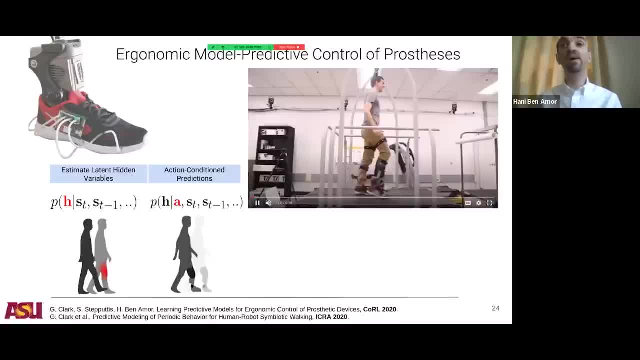 And so what we did in our work is to apply again the same principles of spatial temporal inference in order to have a prosthesis. So that's what you see here: a robotic prosthesis that is able to generate a natural gait for a human user. 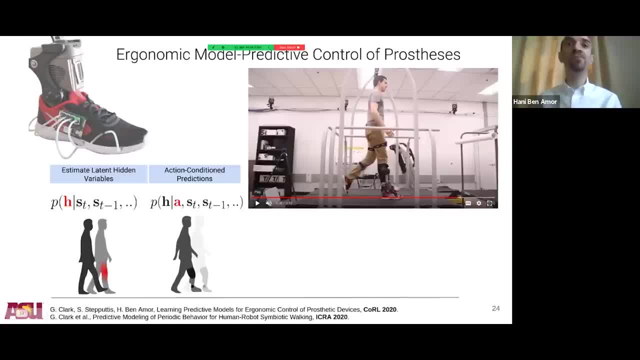 And so what the prosthesis is doing is trying to figure out what should be the ankle angle based on the human's input and the human's motions, And the way it does that, and this is really the new twist that we introduced in our prosthesis. 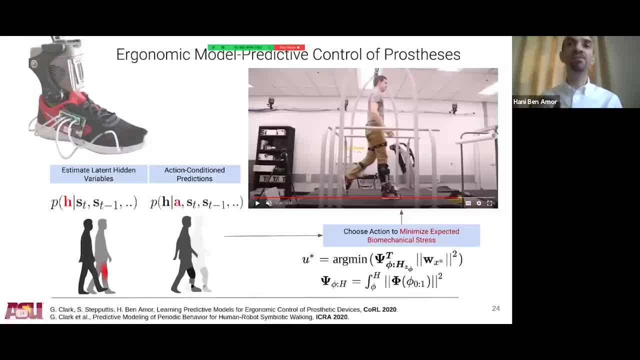 it tries to choose actions by minimizing the expected biomechanical stress. So having this ability to predict into the future, which our framework provides, we are able to predict how much physical stress is there going to be on the knee And we can choose robot actions. 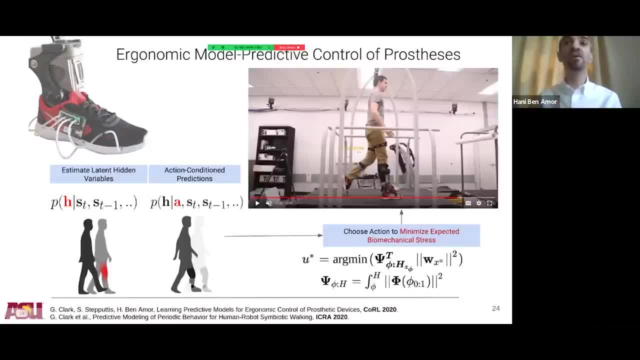 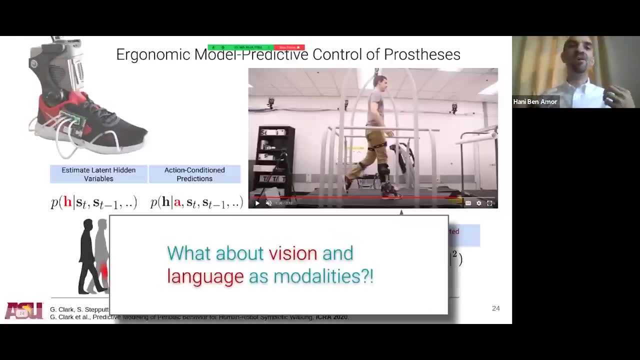 that minimize the stress and lead to ergonomic and safe robot control. So in these kinds of scenarios, it's important to be ergonomic in that it's biomechanically safe. Now we've talked a lot about different modalities and the importance for multimodal approaches. 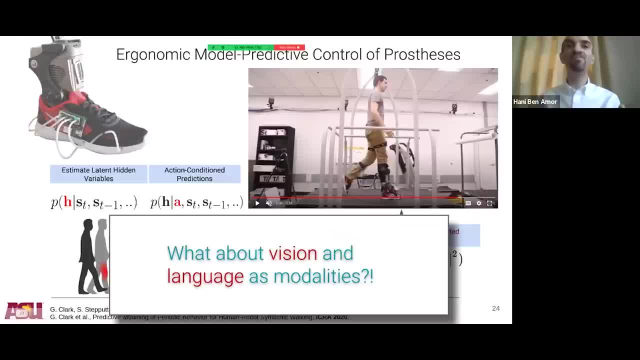 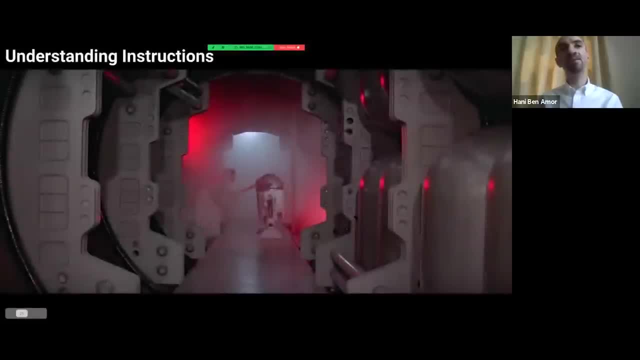 but ultimately, we skipped out on two of the most important modalities: vision and language. So how about those? Well, that's something that I would like to talk about in the next part of my talk. In particular, I'll be talking about 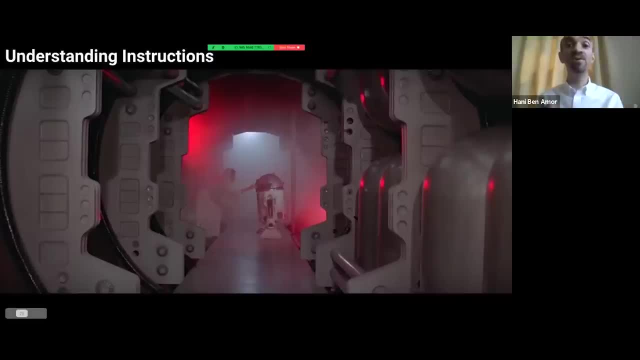 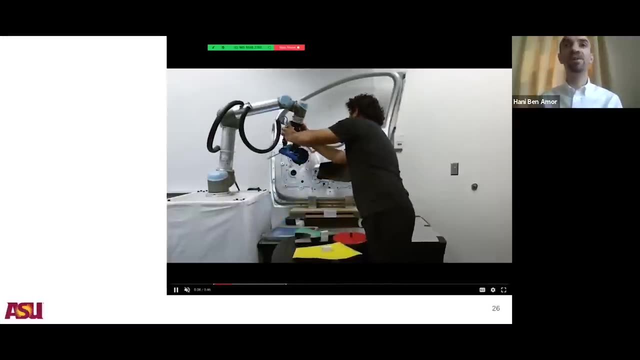 how to understand human instructions and human commands. And so, if we follow the approach that I was mentioning earlier- learning by imitation- we can do a lot of things. So we can, for example, have a user teach a robot how to assemble a car door. 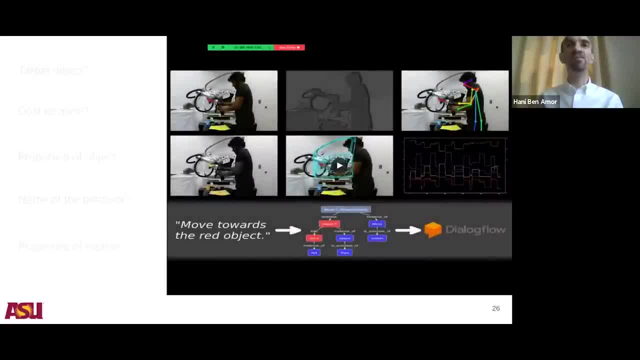 But it's kind of awkward doing it that way, by having a human just move the robot, because there are a lot of things that you cannot convey this way, by just moving things. So this motion domain is not enough to convey, for example, what's the name of the target object. 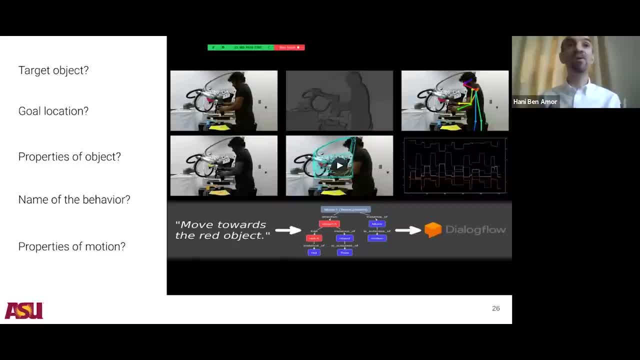 You can't really pantomime that. What is, for example, the goal location? So we need better ways of specifying that. What are the properties of the object? What's the name of the behavior that we're showing right now? What's the properties of the motion? 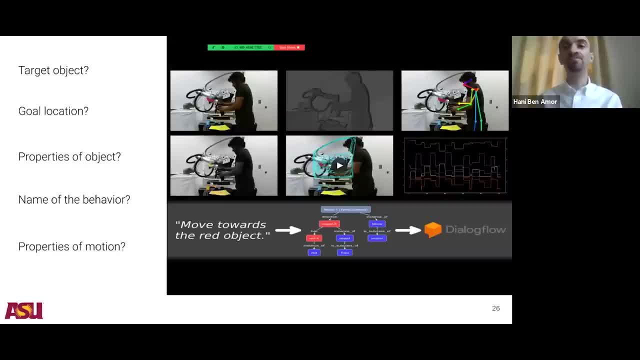 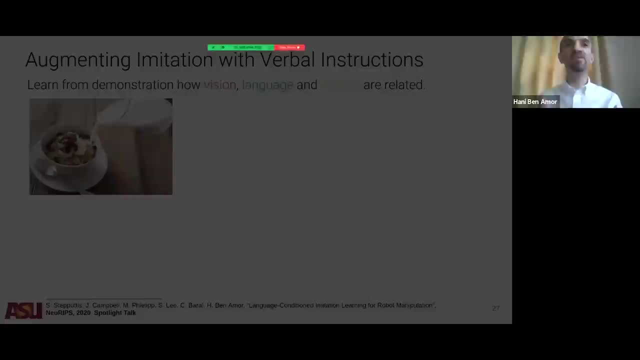 All of that cannot really be conveyed using motion alone, And what we're proposing here is to have the user, as the user is providing a demonstration for imitation, have the user also describe it using natural language, So the user would basically just explain the task. 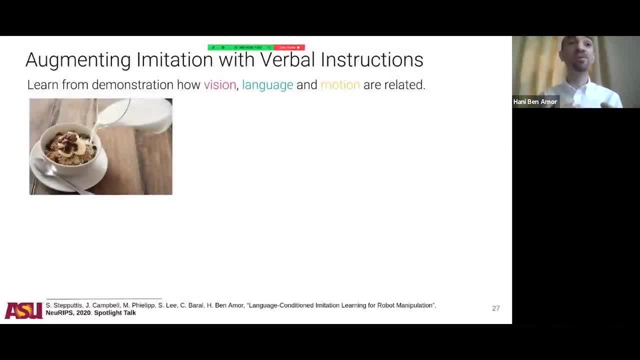 while the user is also demonstrating it to the robot. So think, for example, about you stepping into your kitchen one day and just telling a language or a robot version of Alexa: hey, Alexa, this is how I prepare breakfast. I pick up the milk. 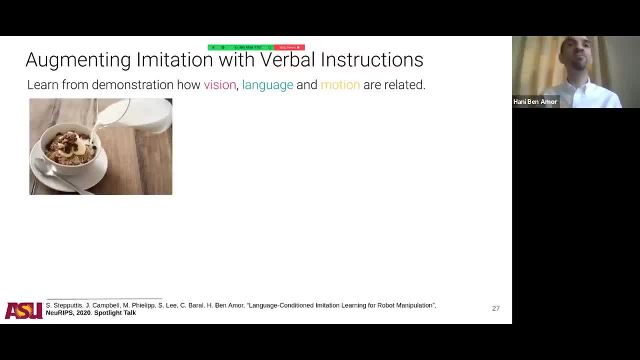 and then you show it physically. So you pick up the milk carton and then you pour it, and then you stir the cereal, and so on and so on. And so, as you're physically demonstrating the task, you're also explaining what the task is. 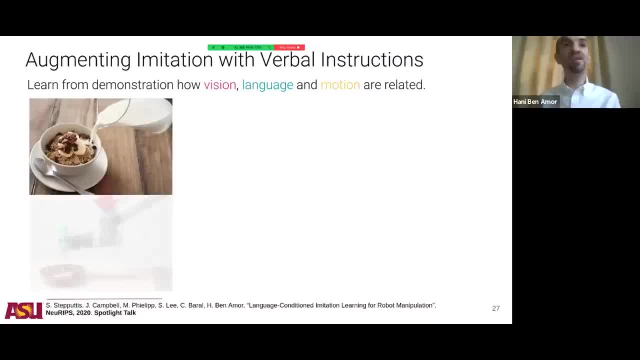 and what the components of the task are, And so, ideally, Alexa would be able on the next day, to actually execute this, and execute this on the robot, And so, in our case, here, what we try to do is to learn what we call a language condition policy. 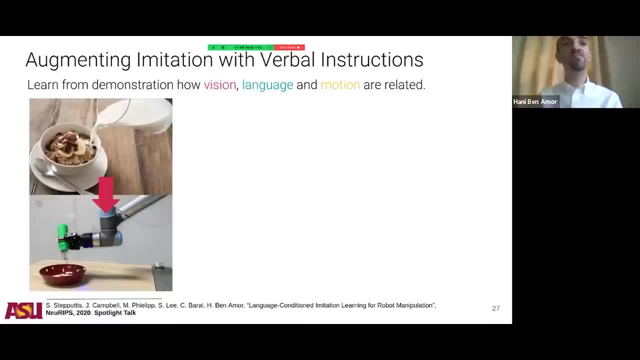 meaning, after we've collected the demonstrations, we can still provide specific instructions to the robot and change what the robot is going to do At training time. we have access to vision, language and motion, So we have a camera feed. We have the natural language description. 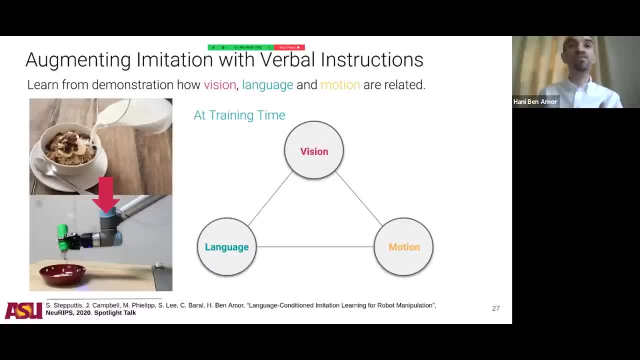 of what the task is, And we have the physical demonstration of what the robot should be doing. So that's available at training time. Now, at test time, what we need to be doing is to only use language and vision. So at test time, 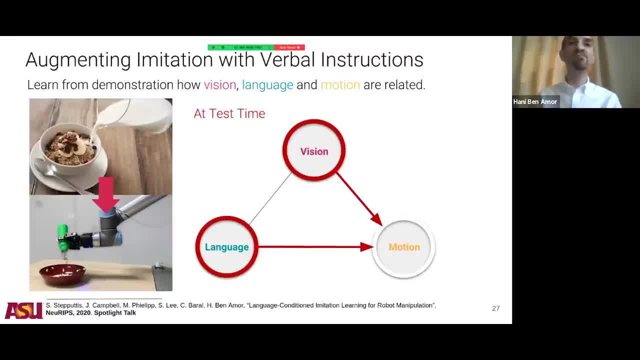 the robot has maybe a new command: Hey, prepare breakfast very quickly, And maybe the robot can also see what the current table layout is. But the robot doesn't know what kind of motion it needs to perform, And so you can think of that. 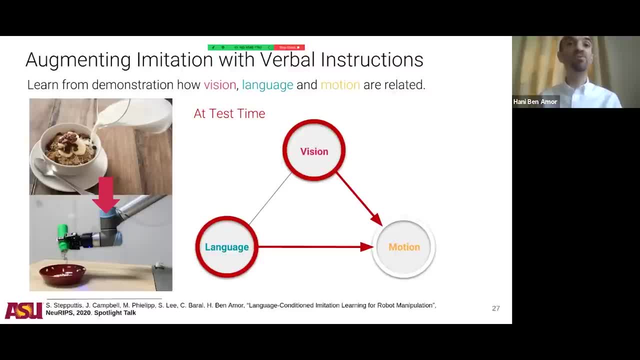 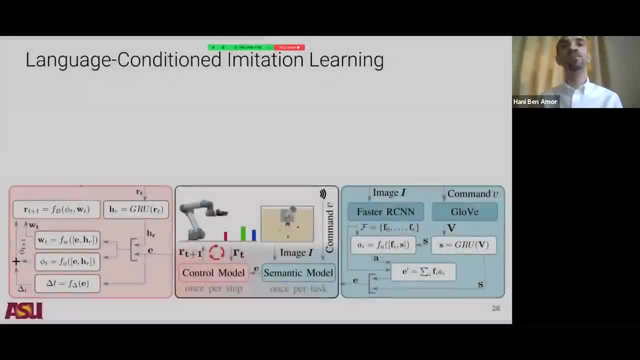 really as a translation process. The robot now needs to use the collected data and the extracted model to make a translation to the motion domain, And so that's what we do in our framework, our methodology that we call language-conditioned imitation learning, And the nitty-gritty details. 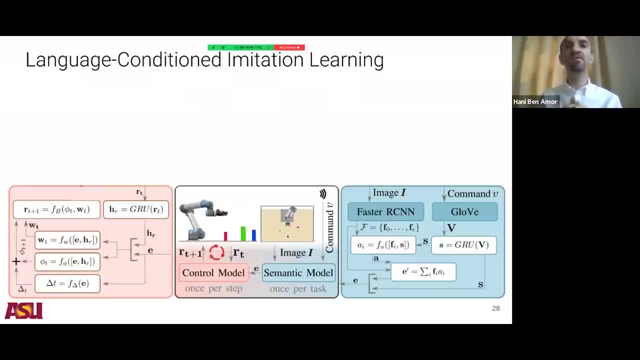 are not really important here The technical details how we do that, But ultimately it's a big neural network that has a component in blue here that processes an input image and a command- a language command as input And it generates as output. 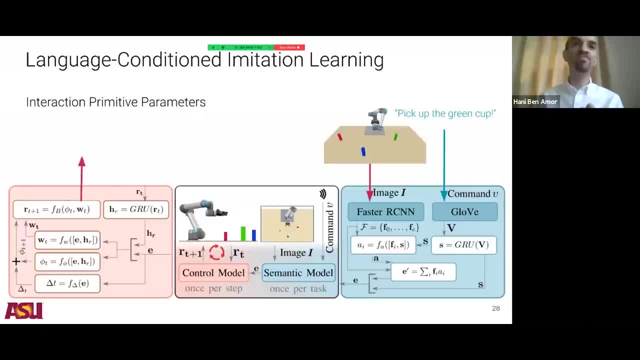 the control parameters for the interaction primitive And the parameters are exactly the parameters you saw earlier: The phase, the phase velocity and the trajectory. So in other words, it's a translation process from image and language to control. Now how do we get data for this? 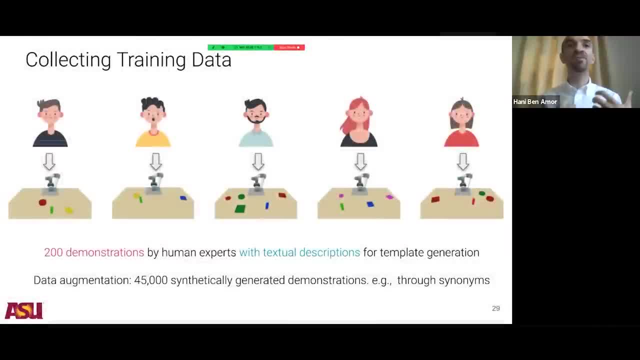 Well, in our case we asked subjects- kind of human experts, you could say, to provide demonstrations. But I want to be honest here. These are not exactly human experts, These are just students that I found in the corridor. So we asked students. 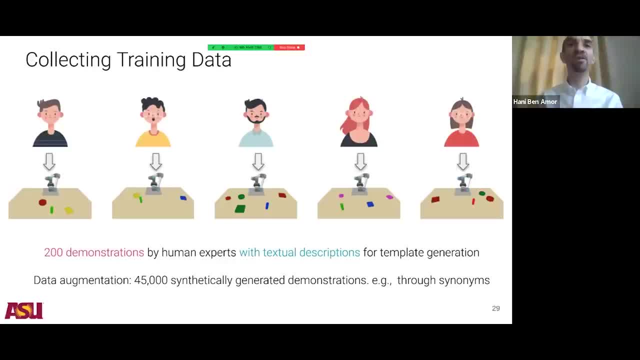 to provide 200 demonstrations. So they would teach a robot how to do something And they would annotate these demonstrations with textual descriptions, So they would write down what actually is being performed right now. And then we also take those 200 demonstrations and then we inflate them. 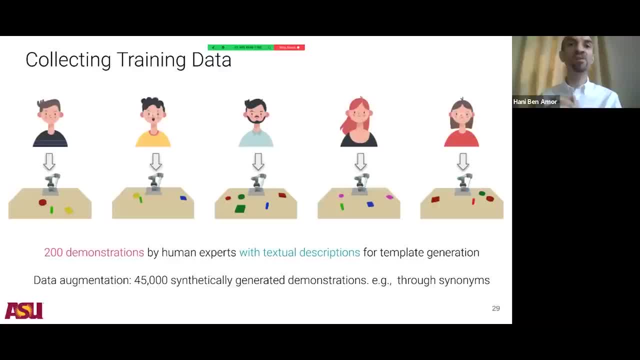 or do a data augmentation to get 45,000 synthetically generated demonstrations. Now you may be wondering: how do we do that? Well, it turns out in language. it's rather easy to do that. You can take a sentence and you can replace words. 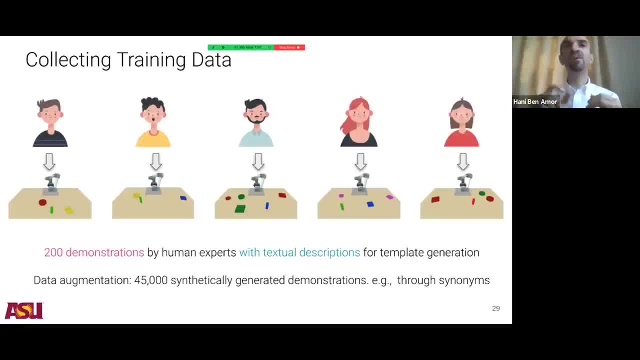 by their synonyms. So if you have a sentence that says pick up the large mug, we can also say pick up the big mug. So basically just replacements of synonyms. OK, so here's now the final network It takes as input: 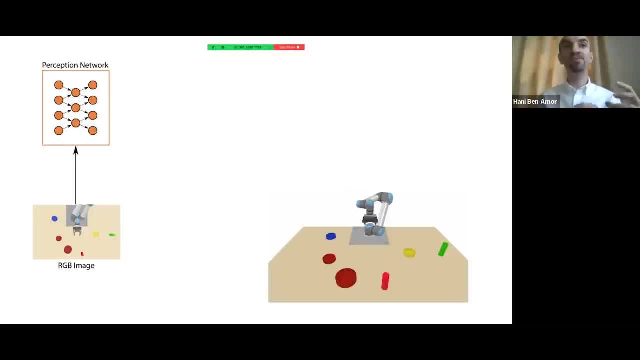 a camera feed. It processes that in the perception subnetwork. It also takes as an input pick up the green cup, a command that goes through a language subnetwork. Then the results of both of these go into an attention network that extracts. 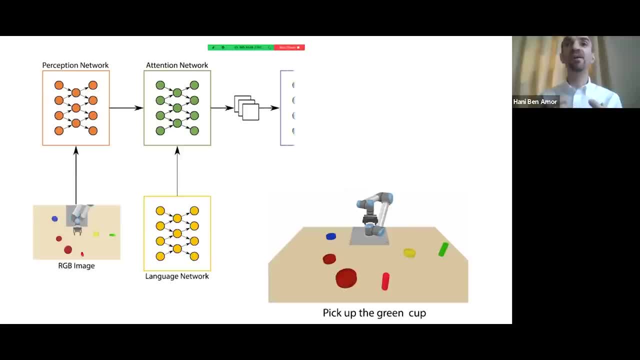 a low dimensional vector that describes the task, That goes into a policy network that now generates the motor primitive parameters And once we have the parameters, we can just run them on the controller, on the robot, and the robot executes the task that we actually gave it. 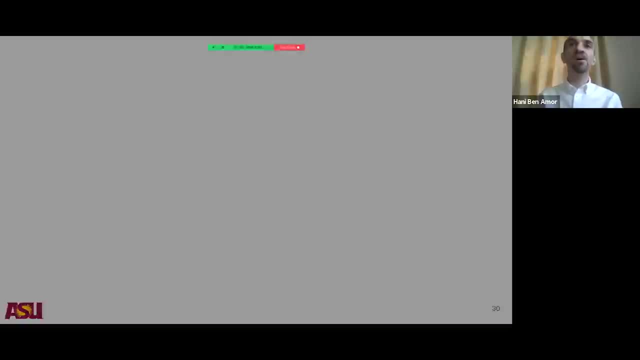 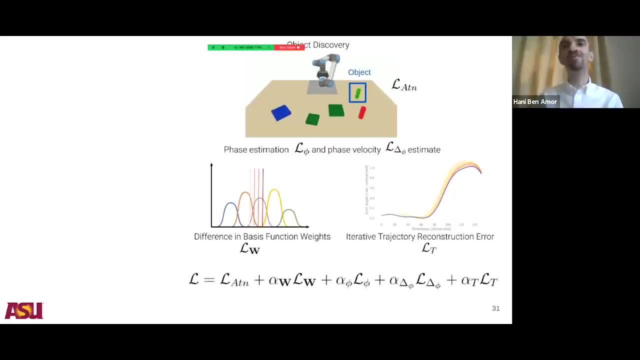 using the language command. OK, so here are a couple of nitty gritty details on the training side. This is only for the experts among you when it comes to deep learning. So in our case we have a rather complex cost function. So that's the L that you see. 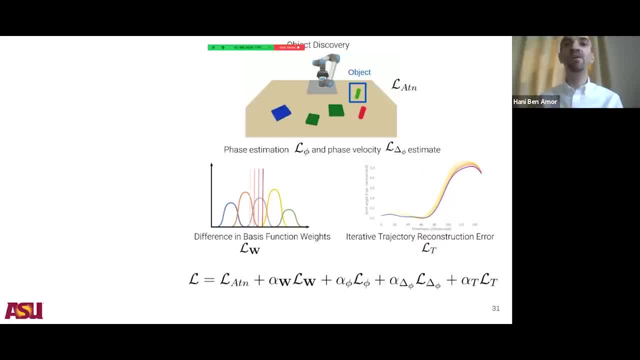 there at the bottom. The cost function has multiple components. Some of these components are related to the object or kind of. what kind of object is in the scene? You can also say related to the visual part of the image. Some components are related to the phase variable. 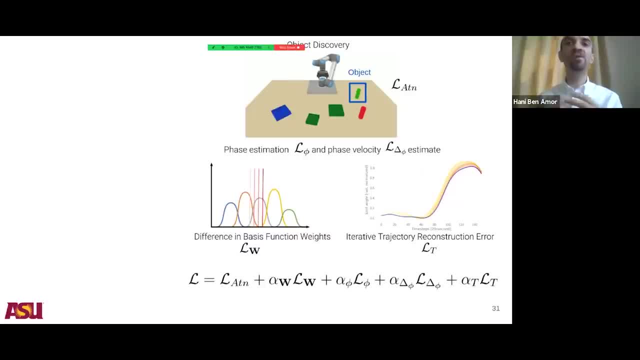 so the temporal part. And then there are some components that are related to the trajectory reconstruction error. So how faithful is the movement that the robot reproduces at the end? OK, and so it turns out, if you don't use a relatively complex cost function. 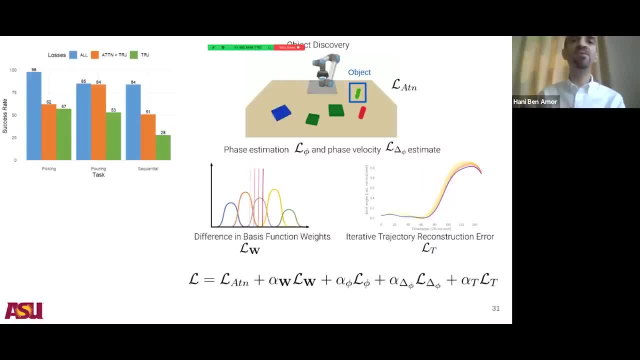 then it can be tricky to achieve success here. So the cost function that I have here at the bottom is what you see in blue, And with that cost function we get 98% accuracy or success in picking, pouring or sequential tasks where you're doing. 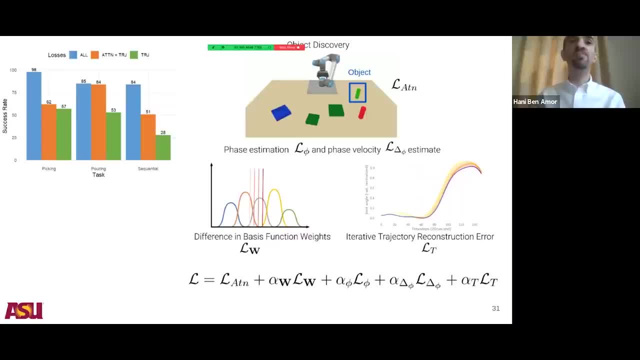 picking and pouring in sequence And if you change something in the cost function you can see significant decline in the performance. so from 98 to 62, which basically indicates that we need to be really careful here in what kind of cost function we choose in training this. 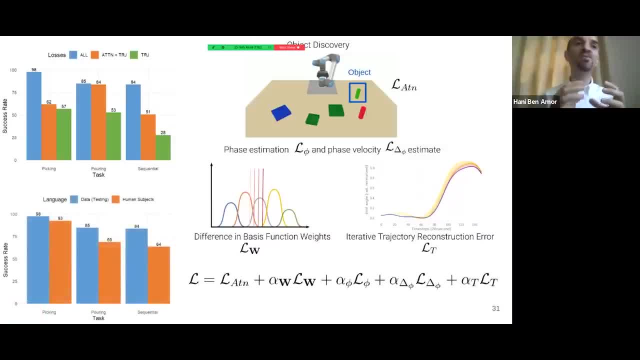 Similarly, we also did a test where we looked at how well this generalizes to new human partners. So if a new person comes in and maybe that person explains the task differently, what the language model generalize to that? And so in the case of the picking task, 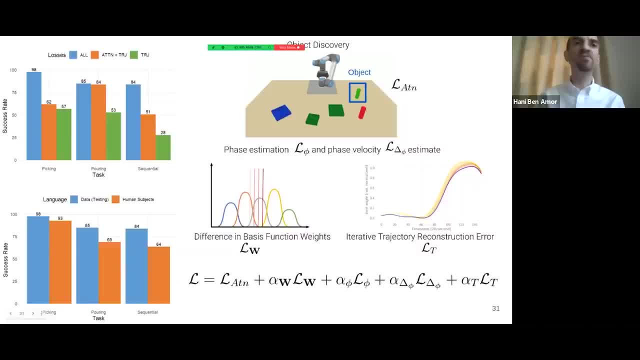 we actually saw that. yeah, it kind of generalizes really well. Maybe there's less variety there of how people can express picking, But in the case of pouring, people use different words and verbs for pouring, And so as a result of that, 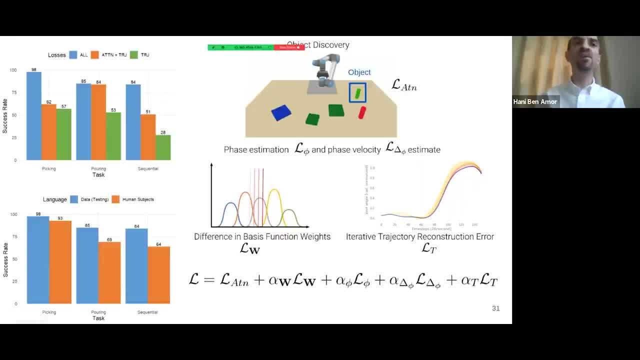 we saw a substantial decline. So now only 69% of the tasks we actually were successful in translating the humans command into robot actions, which means we still need to put a little bit of effort into language generalization. And just to highlight that: 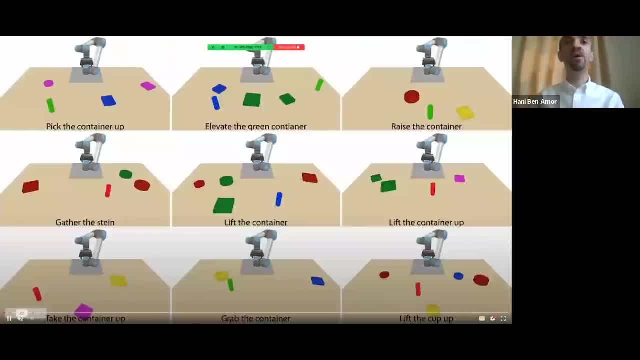 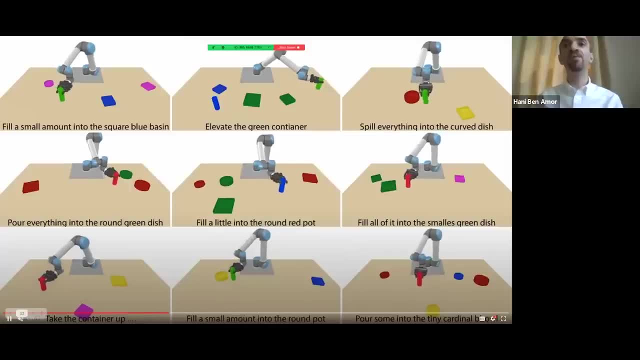 here's a video where you see different ways of different commands that were provided by a user. For example, lift the container, or elevate the green container, or fill all of it into a small green dish, or spill everything into the curve dish. So people may have different ways. 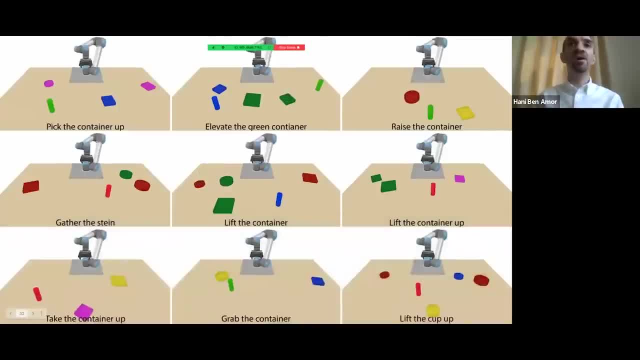 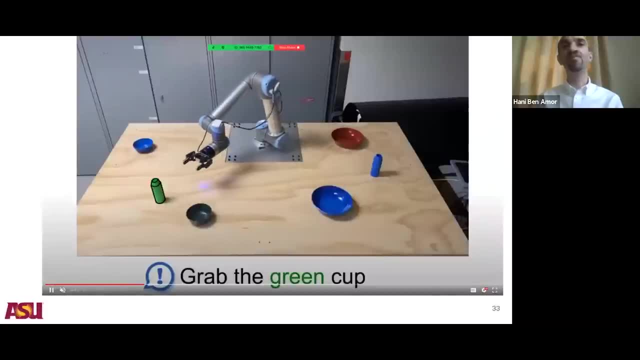 of expressing the same thing. So of course I had to do this on the real robots. So we executed all of this on the real robot, And so now you have the ability to really just step up to it and say, hey, can you do this for me? 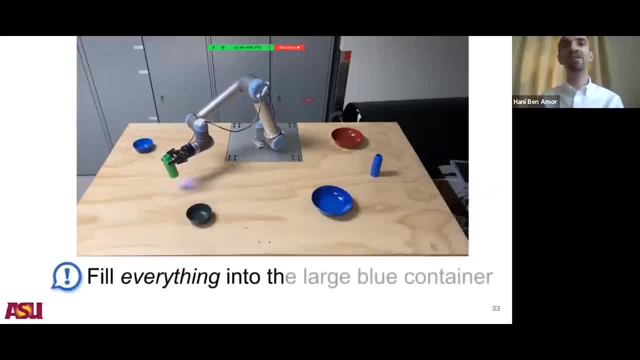 And then it executes that. And here in this example you'll see, even that accounts for small modifiers. So if you say spill everything into the large blue container, it uses the word large to disambiguate which container is being meant here. 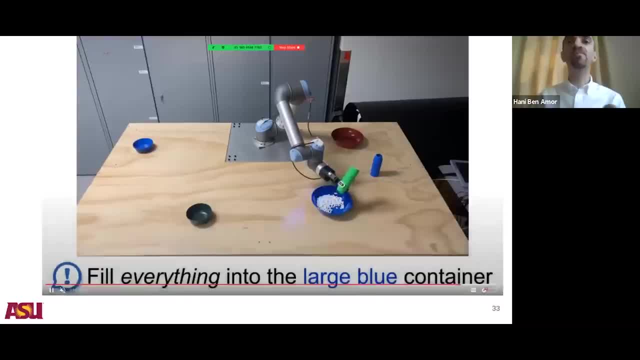 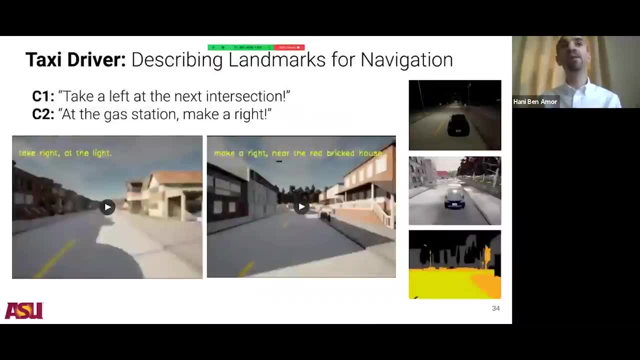 Similarly, it can also figure out whether you're saying: pour all of it or just a little bit into the container. Recently we also applied this to a scenario where you're basically giving commands or instructions to a taxi driver. So think about you sitting in a taxi. 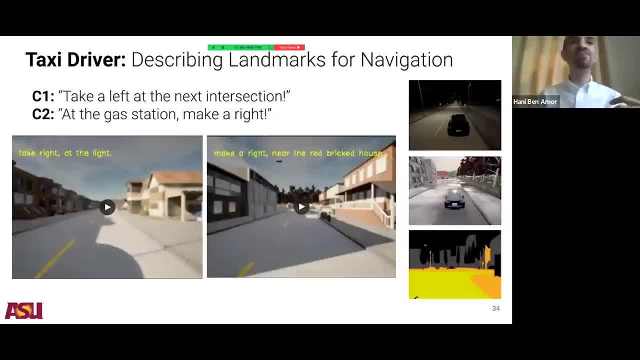 and telling a taxi driver: hey, take a right at the light. And so now the taxi driver is driving, And then, when there is a light coming up, the taxi driver says, OK, now I have to turn right. So that's why we saw the light. 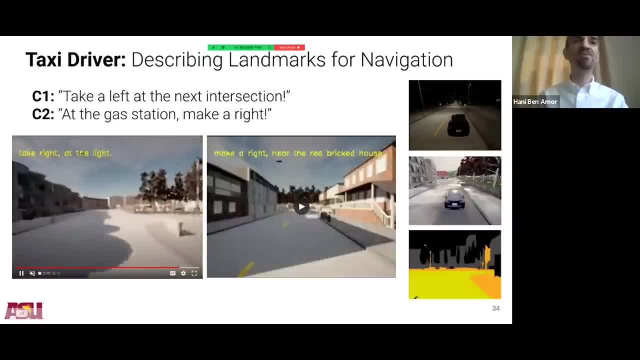 So at the end here, let me just stop there. So there was a light there, And so when our neural network saw the light, it actually said: OK, now I have to turn right. Similarly, here in this task, we're saying: make a right. 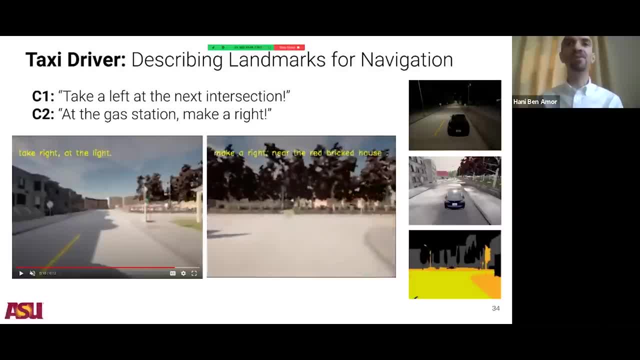 near the red-bricked house. So it saw, OK, there was a red-bricked house, and then it turns right. So again, we're using these verbal commands to actually identify from the scene landmarks And then translate all of that into commands for a robot. 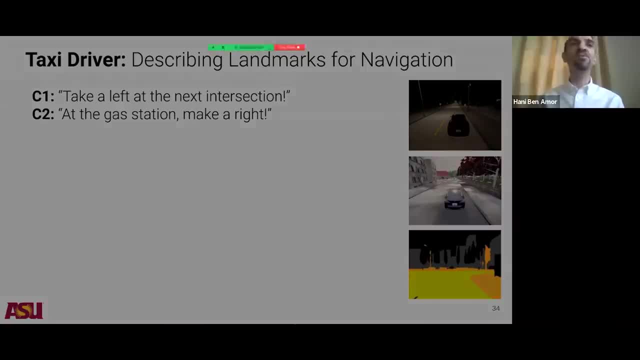 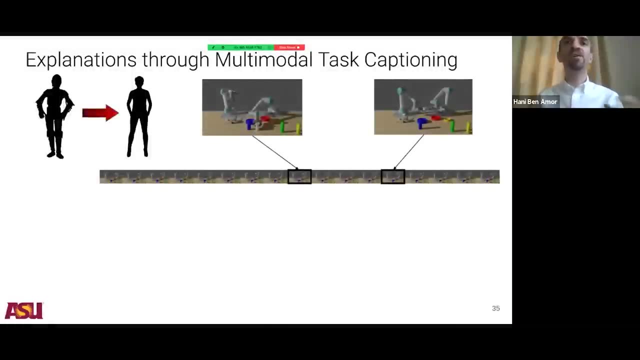 Recently, one thing we've been also exploring is how to have a robot explain something back to a human, And so you can think of that as some sort of captioning process, where the robot is trying to explain what it just did, And so it takes the camera feed. 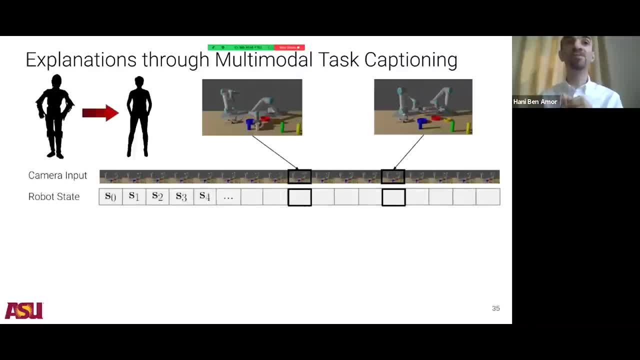 and it also takes its internal states, the robot states, and tries to translate all of that or caption all of that and turn it into a sentence. So, in other words, in this case we're actually going the other way around. We're trying to turn video. 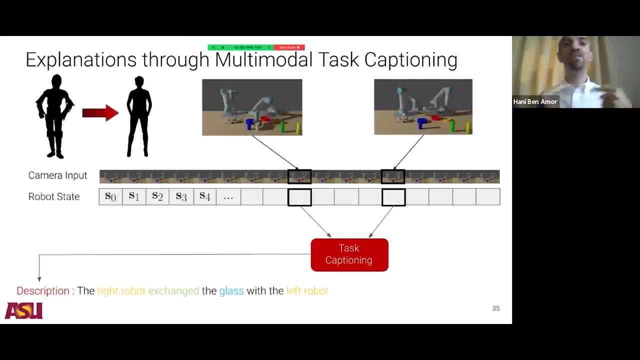 and states into language, rather than language to the states for the robot. And so, for example, in this case the robot may be saying: given what I observed here, the task was the right robot exchanged the glass with the left robot, So a sort of explainable AI. 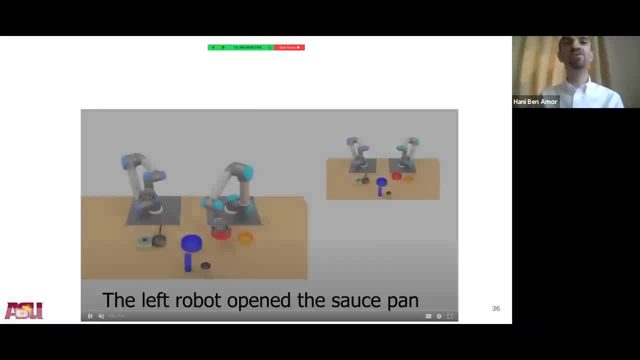 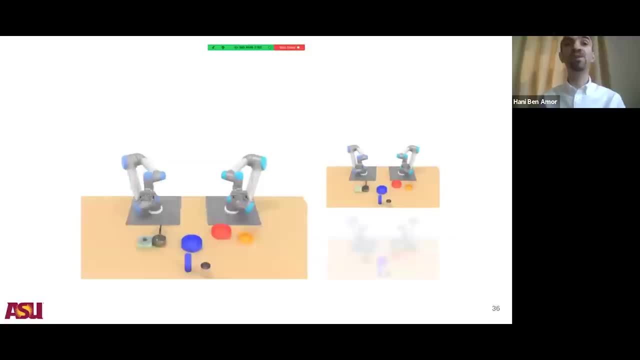 And of course we had to run this then, actually in this case in simulations- but we had to run it. so that's what you're going to see here: One robot executes something, and then we translate all of that to language. So the left robot opens the saucepan. 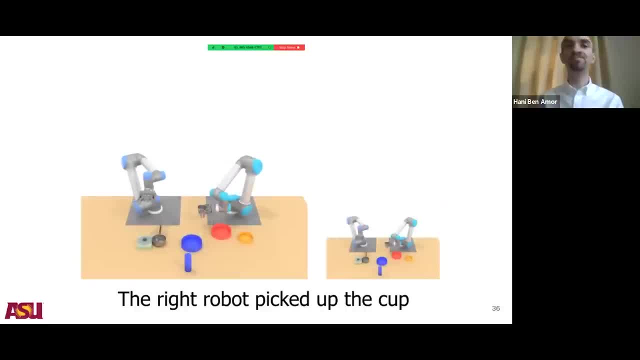 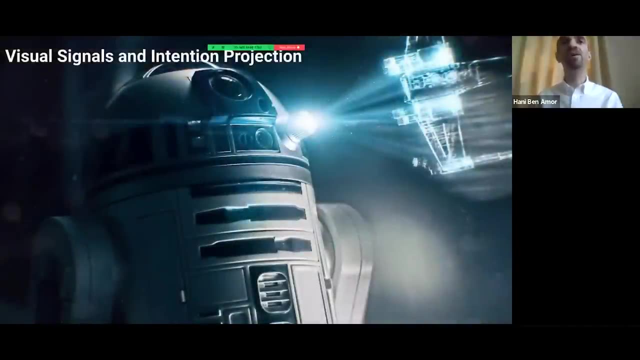 and now the right robot picked up the cup. So that was about language. but maybe there is a different means. Are there other means of communication beyond just natural language? Can we do something, maybe faster, something that communicates things quicker? And so using the Star Wars inspiration again, 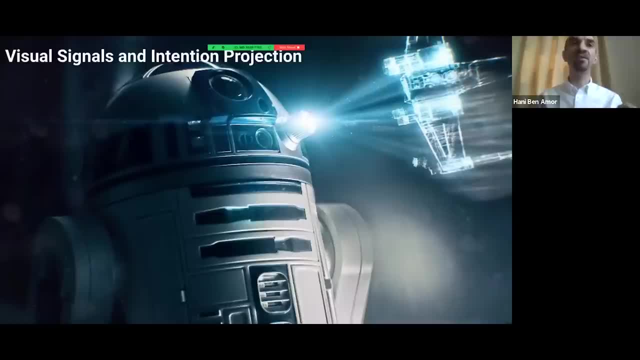 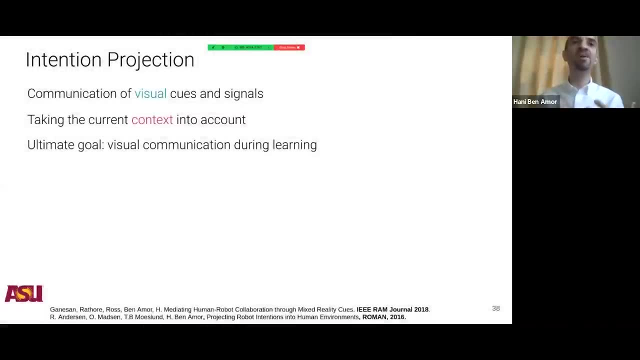 here we're going to be focusing on visual signaling and what I call intention projection. So in the case of intention projection, we want to communicate complex things and tasks and instructions to a human user using visual cues, And the way we do that is by employing mixed reality. 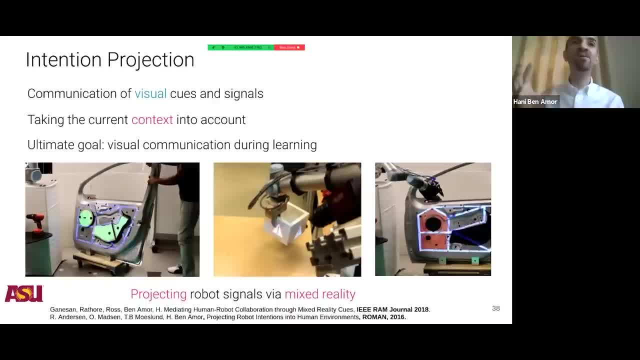 In other words, we're using the context or the environment as a canvas on which we just draw things, And the way we do that is by using a projector that's next to a robot, and the projector projects into the environment information for the human to understand. 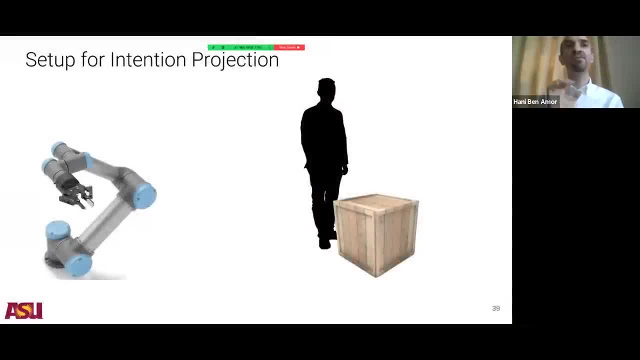 Let me just explain that a little bit more in detail. So this is the typical setup for intention projection. So you have a human and a robot and maybe they need to perform a joint task like lifting a box. Well, in this setup here, 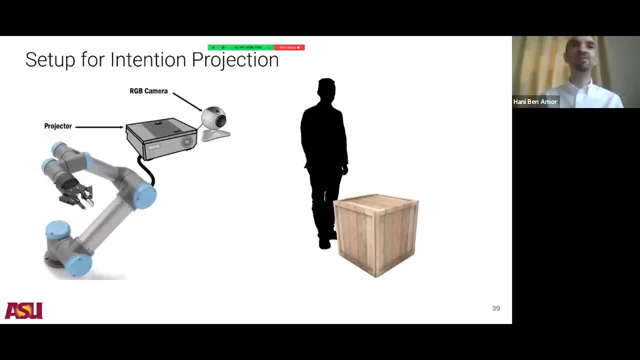 the robot also has access to a projector and an RGB camera, And now with the RGB camera it can detect a box. So it does computer vision to detect the box And it can also track the box in time So it knows what the pose. 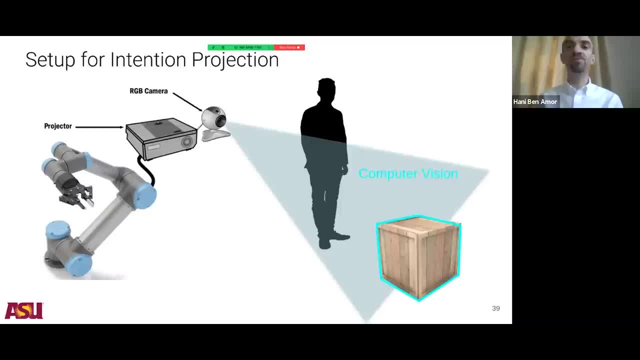 and the position is across different frames. In addition, using the projector, we can project on top of the object information like textures, So you can project on top of the object information for the human collaborator and partner to read. And so that's what you see here. 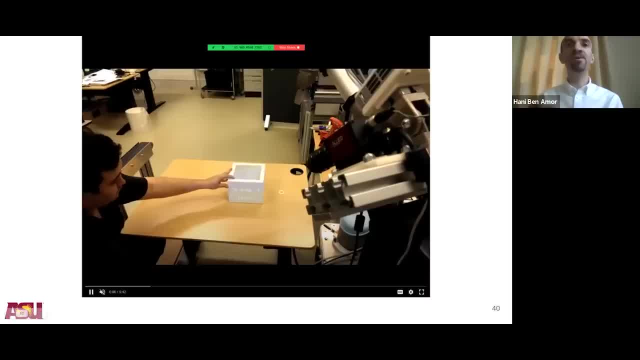 in this video. So, for example, in this case the robot is telling the human to area one, So move this box to area one. And there is this: four centimeters here says how much of a distance is still left And when the person is finished. 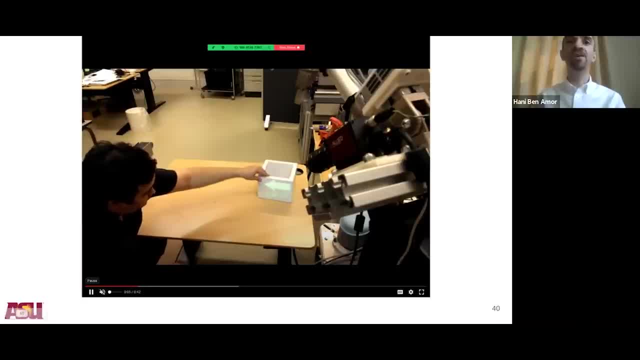 the robot says, okay, rotate the box. Okay, the person is finished again. And now the robot is saying, okay, don't touch the box because I'm going to manipulate it, And so what we want to do here is to ensure safety. 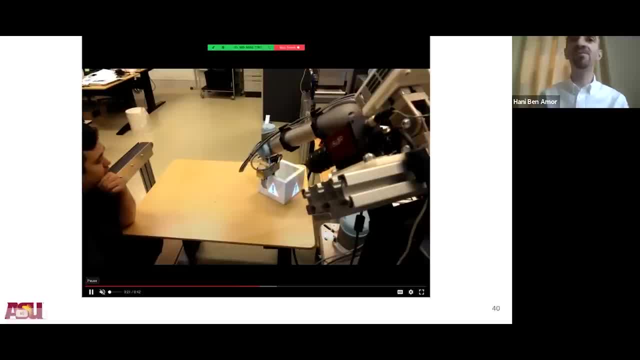 by projecting the safety triangle. Keep in mind that in the setup here we have a camera and the projector. It's what you see in the right there next to the robot. So the robot picks up the box, moves the box and you can see that our projections. 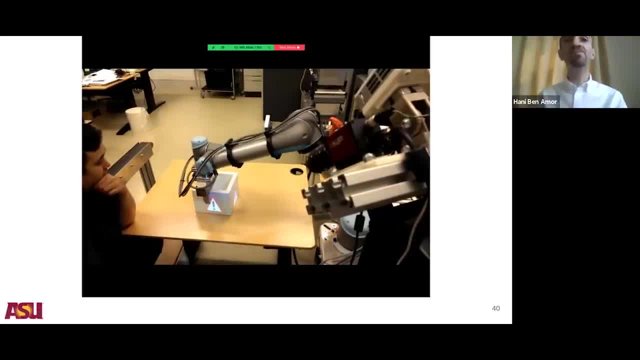 follow. actually Keep in mind that this is mixed reality. So we are not using any goggles, We are not using any head up display or anything like that. This is actually really happening in the real physical space And we're using the projector to draw on the real physical space. 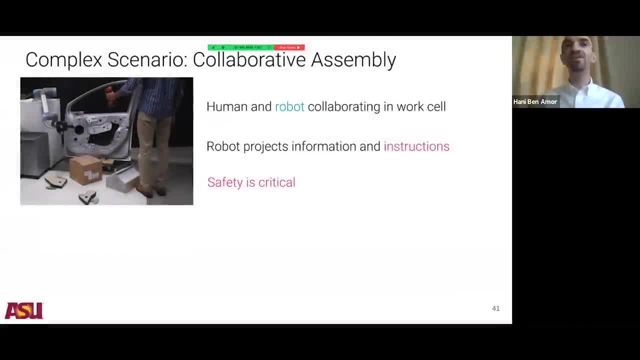 Now you may be wondering: maybe the task was too easy, too simplified. We can do the same thing also in more complex scenarios. So we applied it also to collaborative assembly, where humans and robots have to collaboratively assemble a car door. So that's more complex. 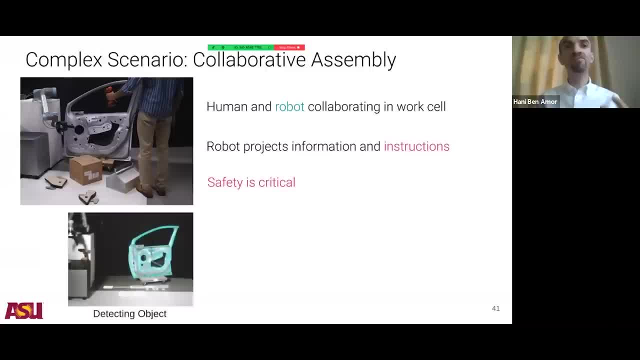 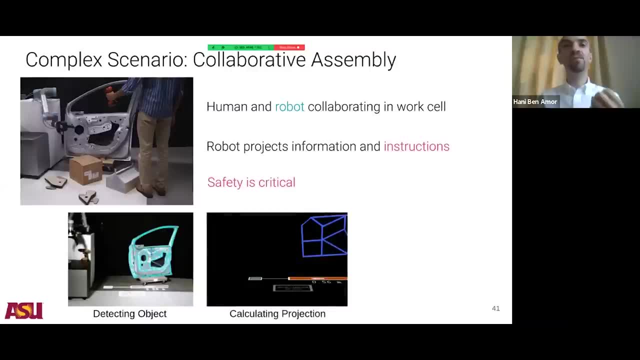 And so, here again, we're using the same methodology. We're detecting the object- the car door in this case- using computer vision, We're tracking it and we're using that information to calculate 3D information which we're going to be drawing. 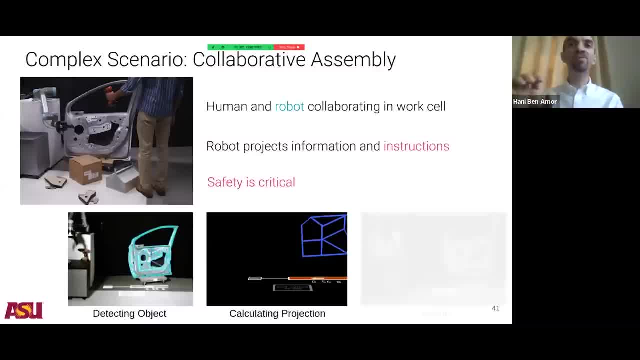 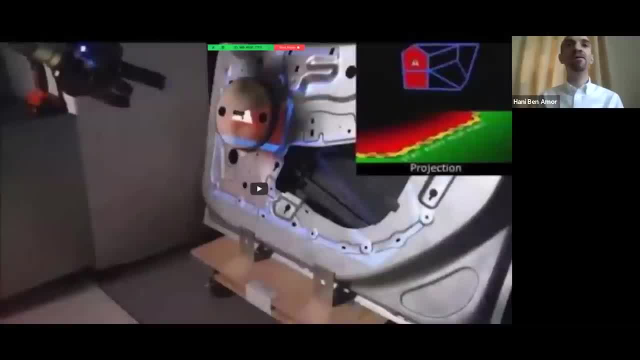 on top of the car door And then, once we project all of this into the real world, we have really the environment as our screen. Okay, here's an example for that. So what you see in the middle is the actual car door being moved. 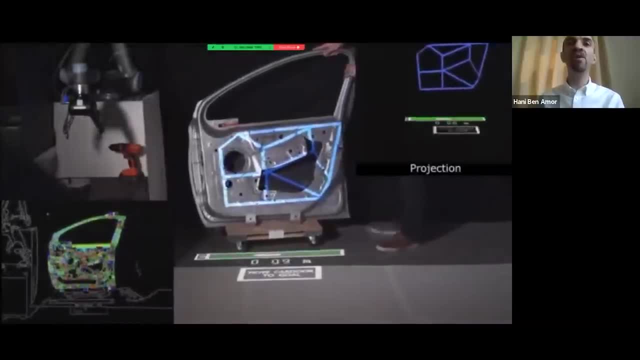 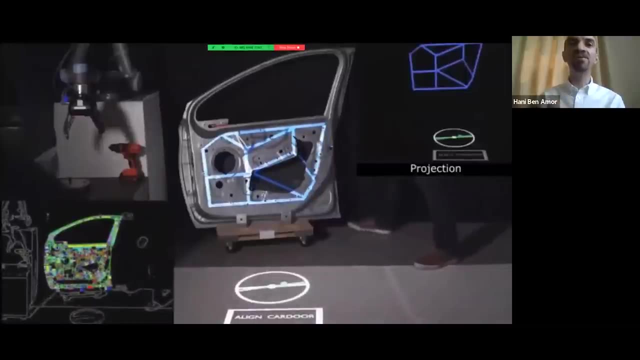 And on the floor you'll see additional information about how much distance is still left or how much the person has to rotate the car door, And so in this case here the green dot needs to go on top of the white dot, And the person can do that. 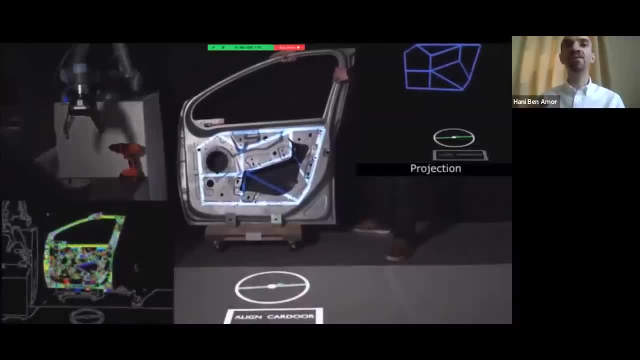 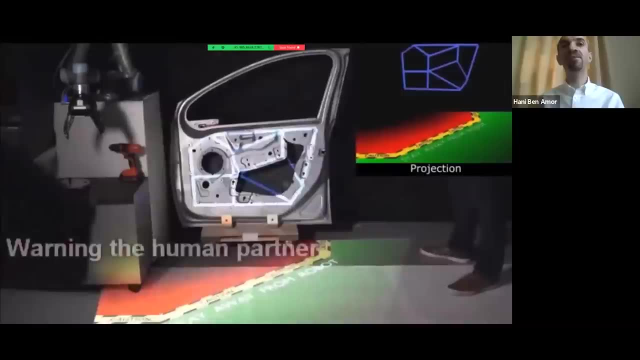 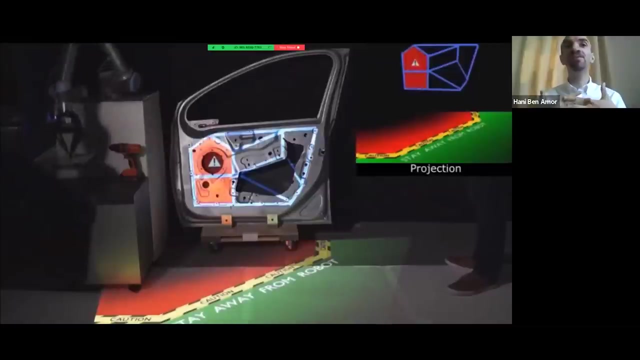 by just moving the car door. So align the car door and the person aligns the car door by moving the green dot onto the white dot. The robot can also project information as sort of a warning about any potential collision or any potential risks to the person. 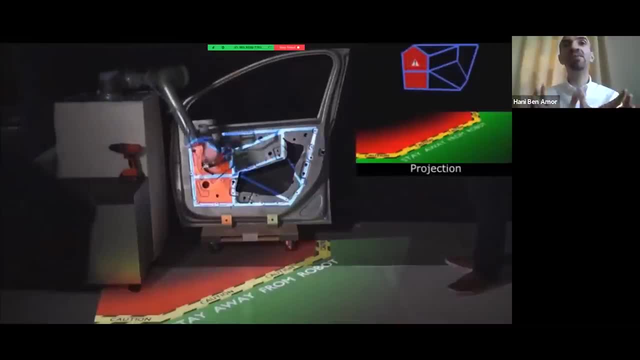 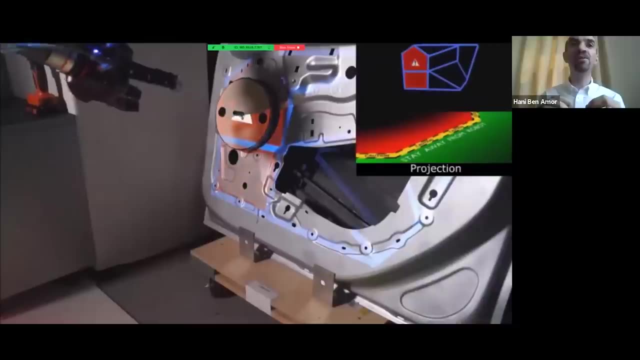 So in this case, here the robot can actually project its safety area, saying stay out of this area or stay away from the robot, And it predicts specifically to the person which areas are safe and which areas are unsafe. Similarly, the robot can also accurately guide. 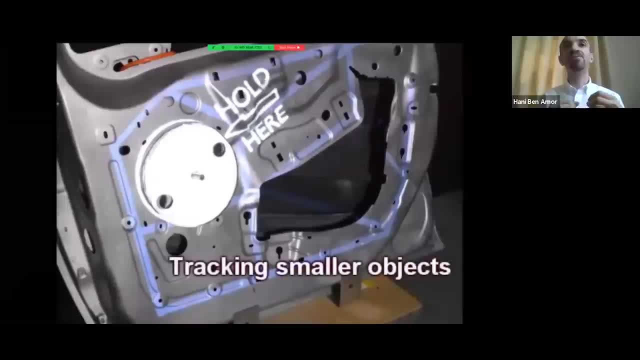 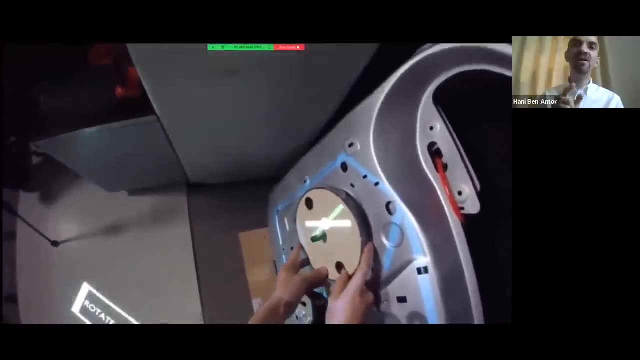 the human throughout the task And so we can project, for example, information saying: hold the object over here and rotate it. So in this case the person needs to align the green line with the white line And when the person is finished, 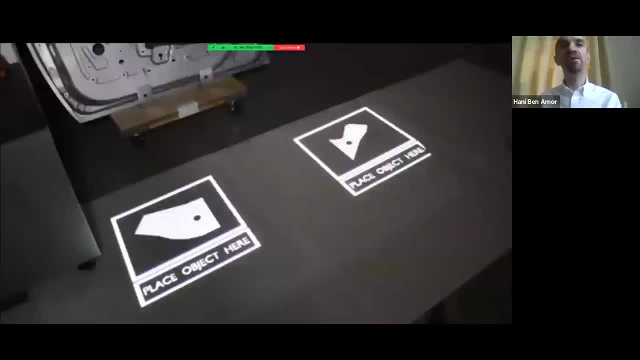 we say you're done. So really think of this as a just in time teaching and collaboration framework where we are providing information by tracking what the person is doing, by tracking what the objects in the environment or where objects in the environment are, and by projecting specifically. 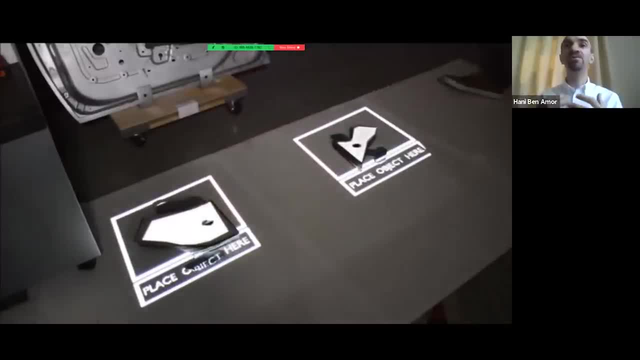 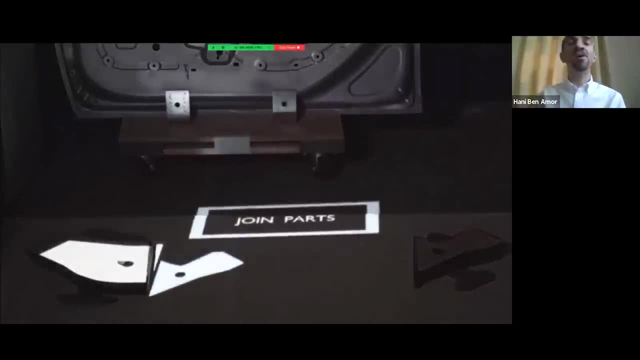 into certain areas in the environment information. So in this case, here we're projecting information saying these two parts need to be joined, And so this may sound like it's very specific to a task, but actually we have shown in one of our papers. 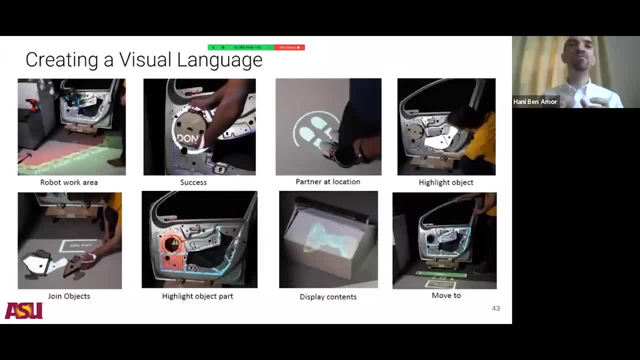 that you can create a nice visual language out of this that allows you to create sentences, kind of visual sentences, by combining the different pieces, verbs and objects and so on and so on and adjectives and so on, So by representing all of that in the visual space. 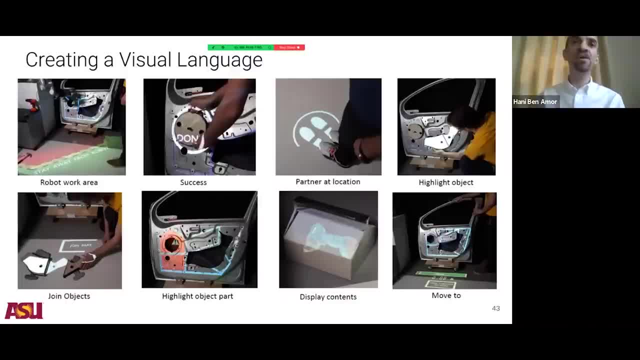 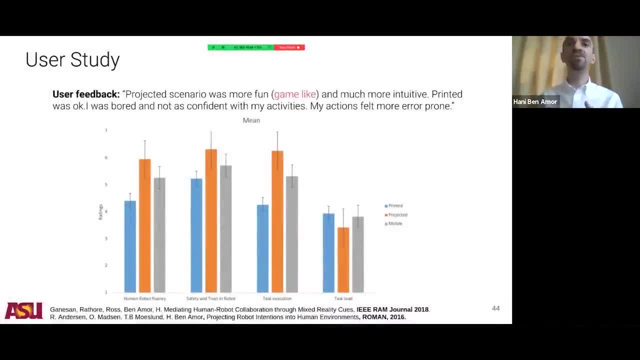 we can create some sort of visual language. And at the end, we also did, of course, a user study where we compared this to a printed sort of a collaboration task where users had just a piece of paper with the task description as a piece of paper. 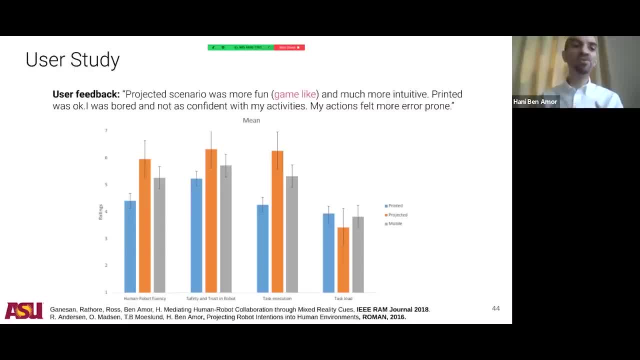 basically just a verbal task description. And we also tested this against a sort of an iPad, where we had on the iPad additional instructions for the person. And so we tried to figure out: does the projection help when we compare it against an iPad with videos? 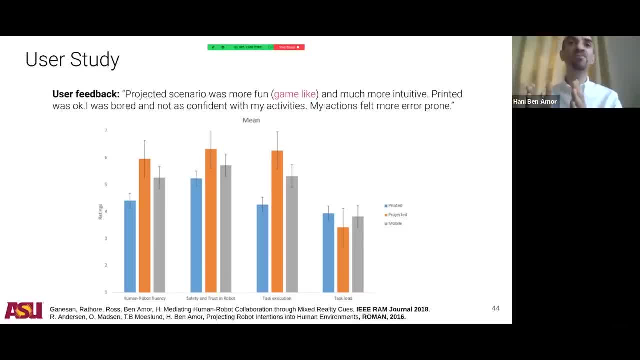 and sort of an interactive description of the task or when we compare it to a more traditional textual description on a piece of paper. And we saw that across human-robot fluency, safety and trust in the robot task execution and task load, we saw substantial improvements. 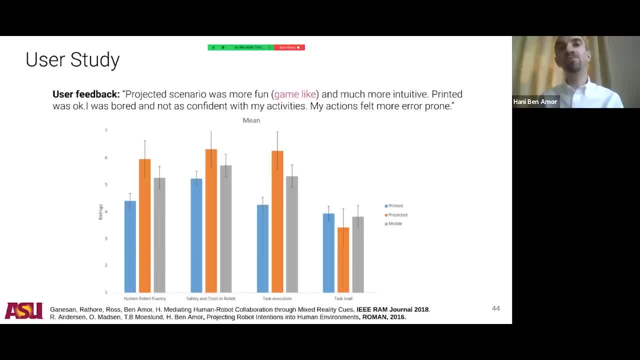 in all of these metrics, But one thing that was really helpful to me in better understanding why people like this is: people actually said that they liked the scenario because it was more fun. It was game-like. So there is this element of gamification in all of this. 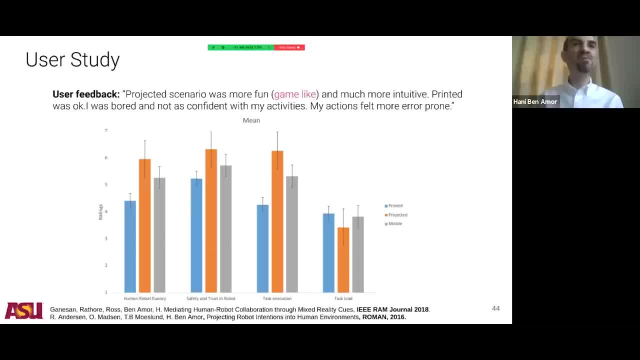 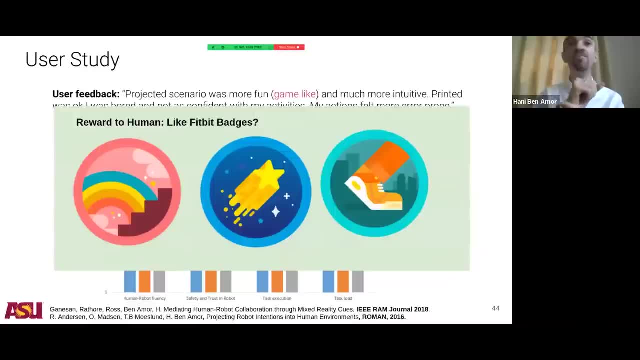 And so you know, there's a lot of things that we can do to make it more fun, And that made me think about this. So, if you think about things like Fitbits and these modern watches- for example, the Samsung watch- 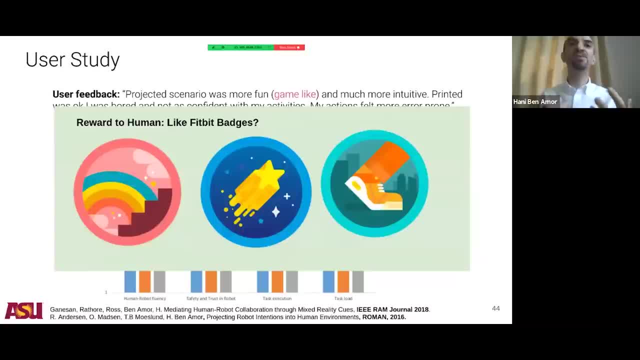 they try to use some sort of visual feedback in order to encourage the user. So in one of these smartwatches nowadays they would show these emblems and these badges to you whenever you go running or you stand up after two hours, And so. 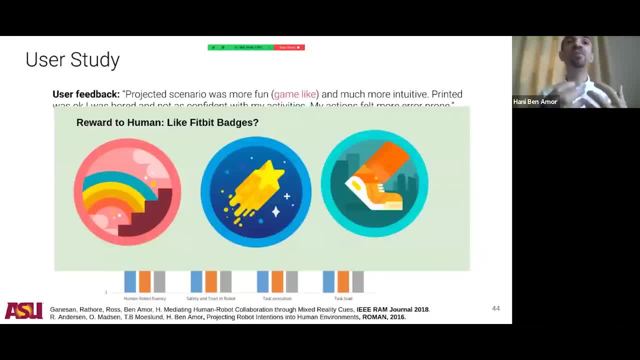 you know you give visually some sort of reward or some sort of encouragement, And so one of the things I'll be investigating next is how to use this mixed reality projection technique in order to give visual rewards to the human user and kind of a guidance. 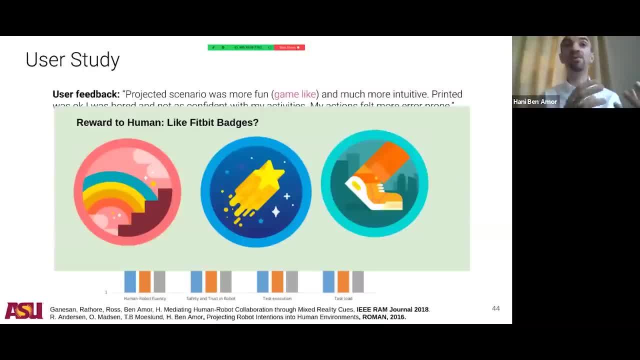 and help the human learn. So not only have the robot learn to adapt to the human, but potentially also kind of reward the human and condition the human's behavior to become a better partner in this collaboration and partnership. And so with that we come to the end of my talk.